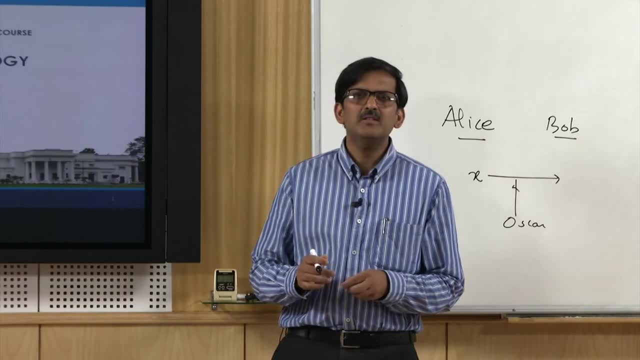 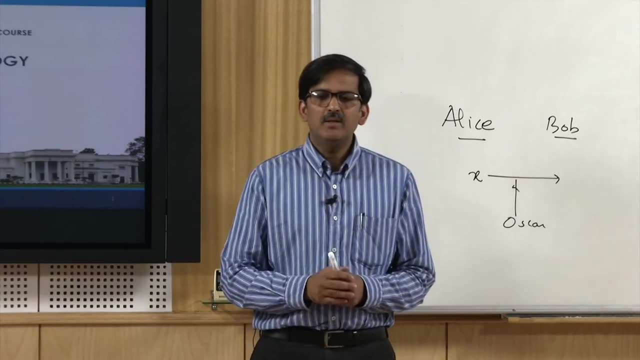 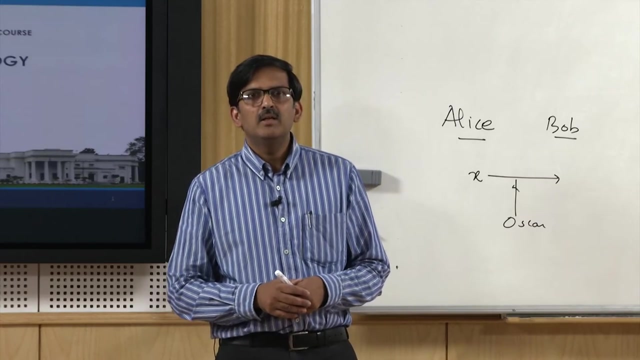 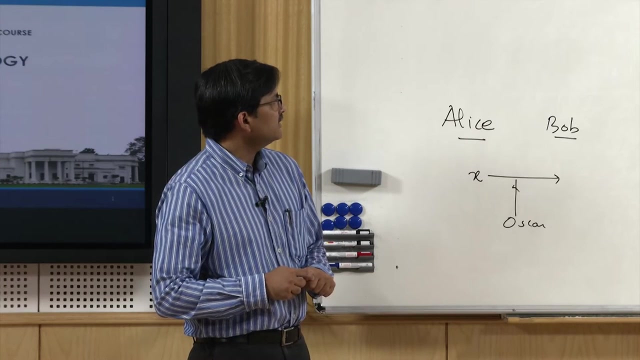 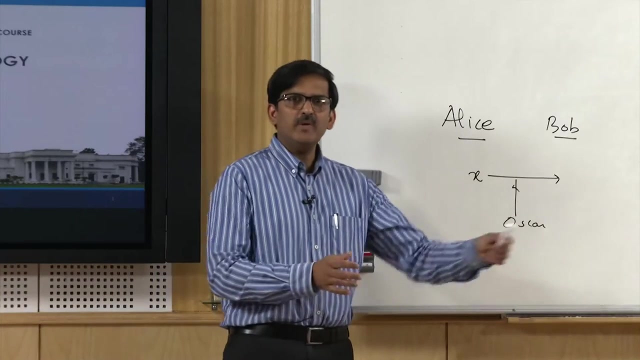 we have quickly also seen the weaknesses of classical cryptography. we have seen block ciphers, So mainly private key cryptography, and then we have seen RSA, which is the public key cryptography. So we have another problem that is somewhat different from communication, At least communication across space, that is, in some way communication across time. Now, 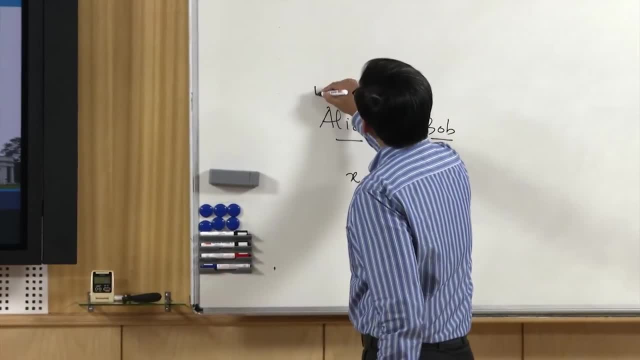 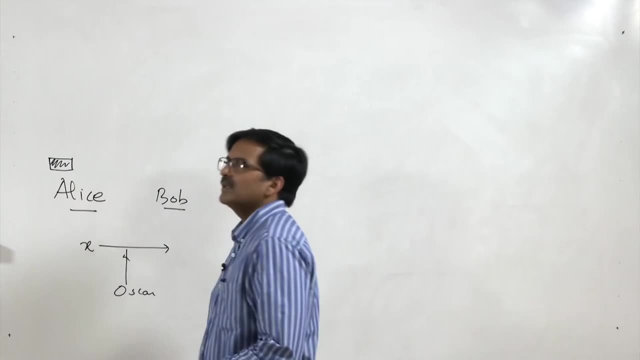 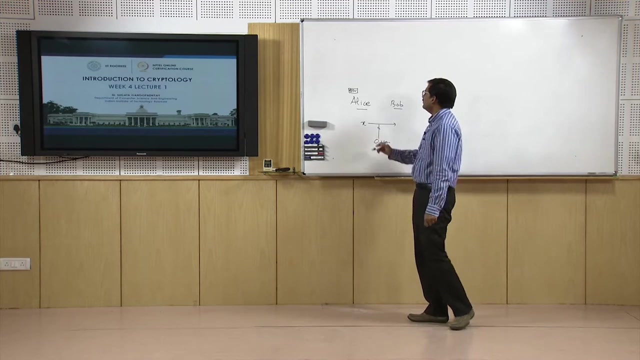 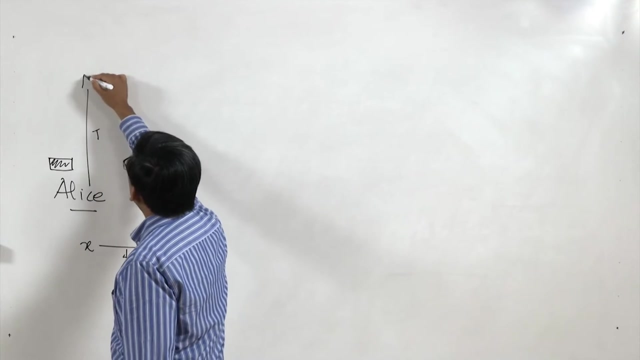 suppose that Alice has an hard disk which she keeps and goes away, and suppose that this hard disk is accessible to more than one people. Now, after some time, back after some time, Alice comes back. Let us suppose after length of time Alice comes back and checks the same hard disk. 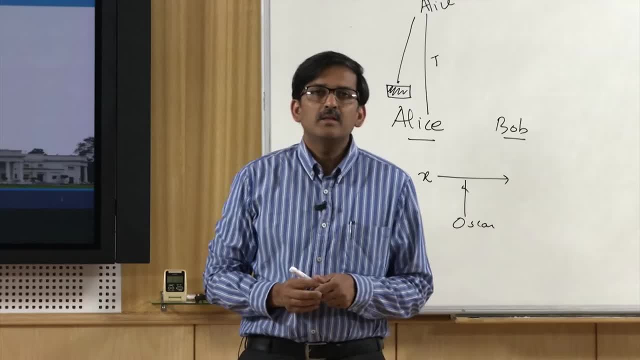 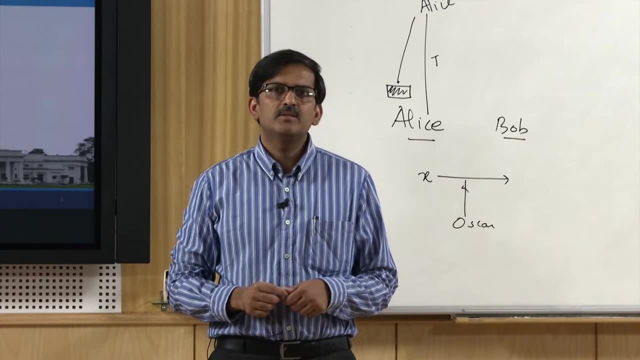 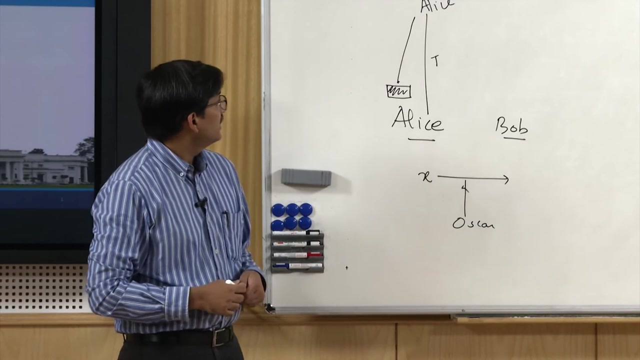 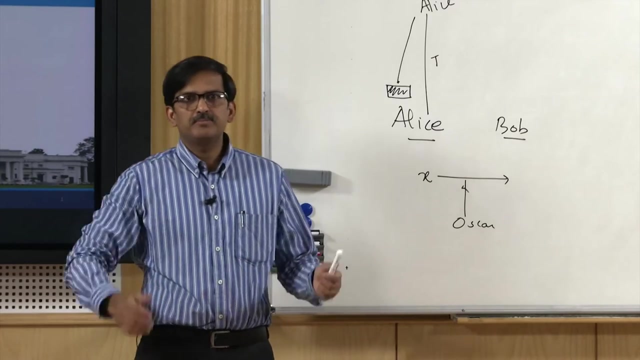 What she asks is that, whether anybody has tampered with the hard disk or not, in her absence. Now our question is that: is it possible to secure this hard disk for Alice, so that at least She is sure whether everything is all right? Now there is another question here, I mean: 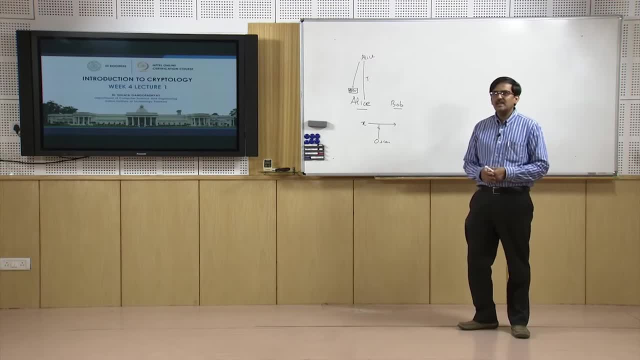 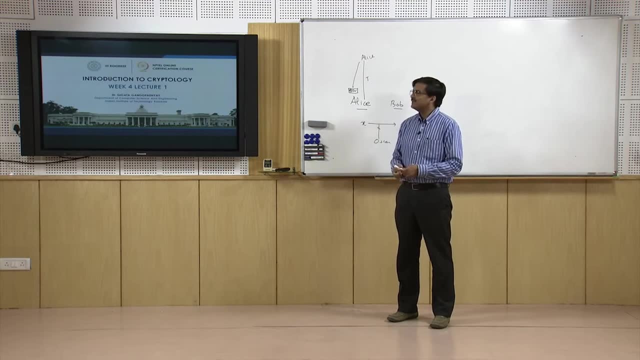 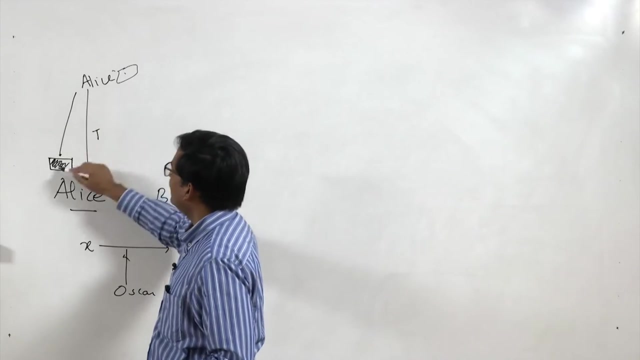 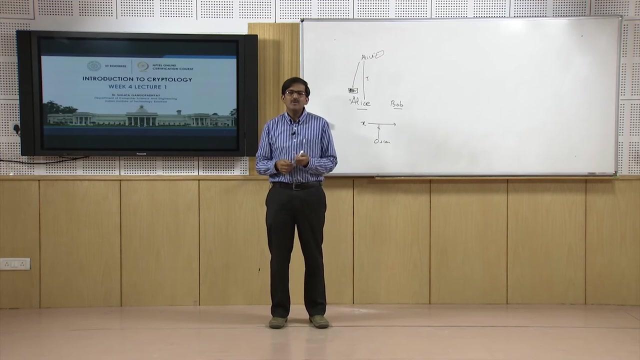 like, or someone might say that of course Alice can do this. Alice can well check a, keep a copy of the hard disk, the whole hard disk, take it with her and then when she comes back she can match bit by bit- Yes, With the bit by bit, the hard disk that she left with the hard disk she has been carrying. 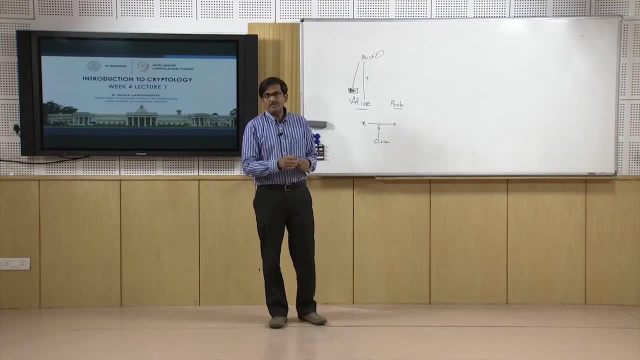 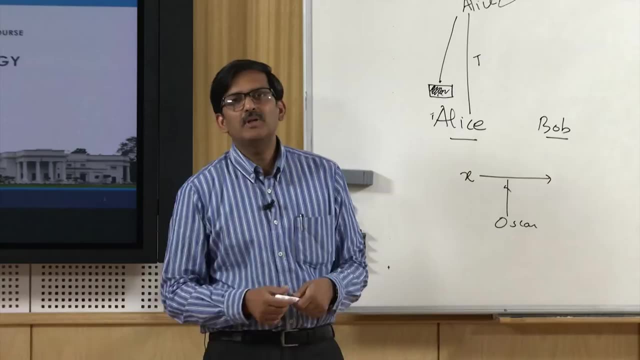 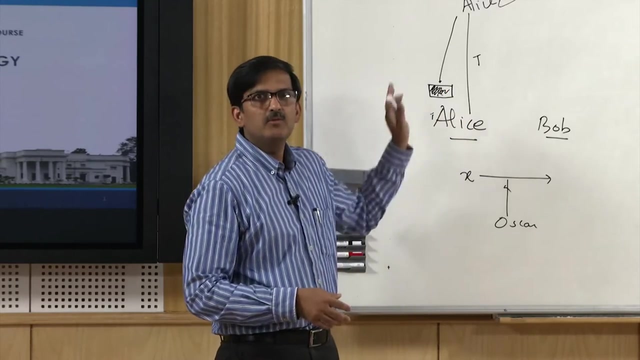 but then it beats the purpose. It does not serve the purpose because then Alice is carrying the same hard disk of same size, so she could have easily carried the whole hard disk from here and removed, I mean whole data from here, and removed whatever is over here. So ideally, 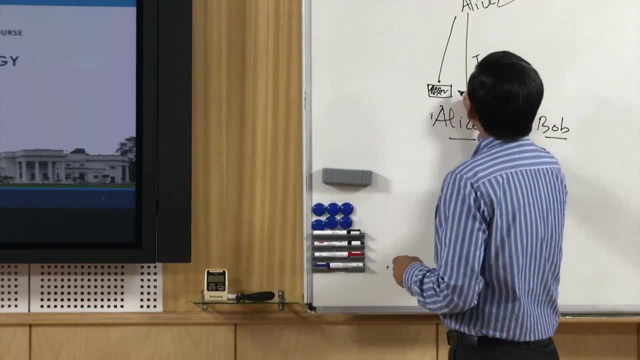 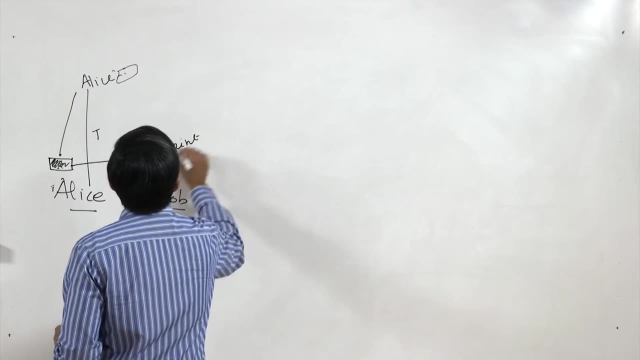 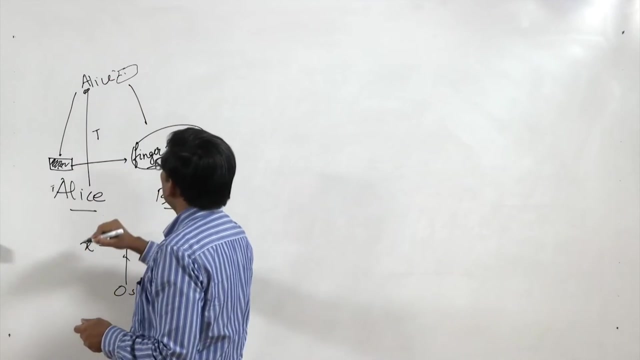 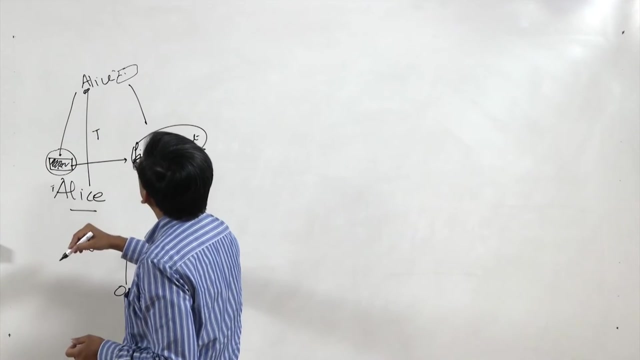 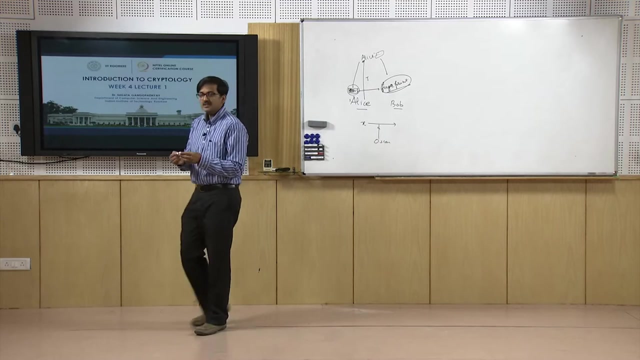 what Alice would like to have is a wing order Right small finger print of this hard disk and carry it with her and when she comes back after some time, calculate the finger print again from this hard disk that she left behind, and if this, these finger prints match, she should be reasonably sure that no one has tampered. 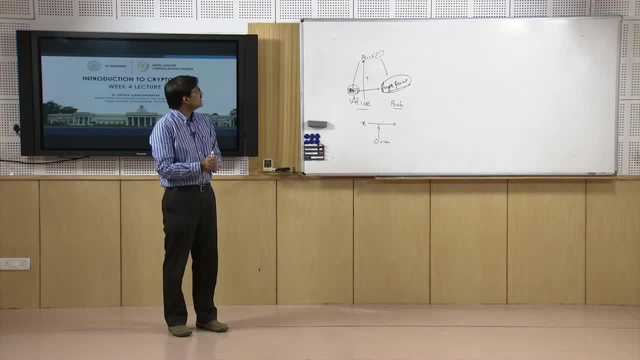 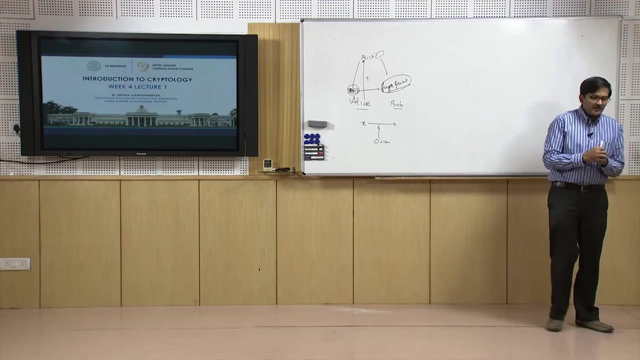 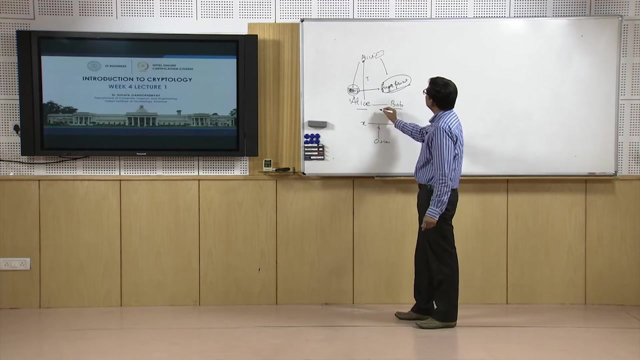 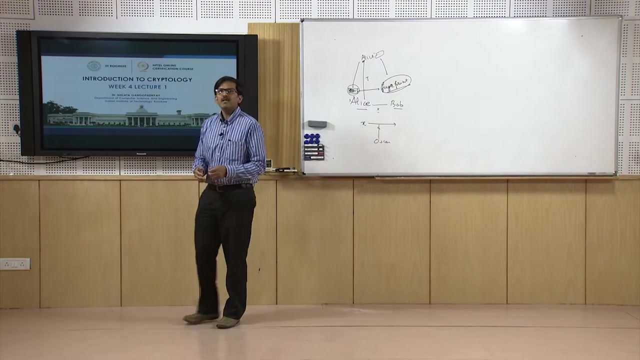 her hard disk. So that is something that we would like to see, whether I mean something we would like to see whether it is possible to do. There is another thing that is important: when Alice is communicating to Bob- suppose Alice sends a message x, now she might be encrypting that message, but still, when Bob gets a message, 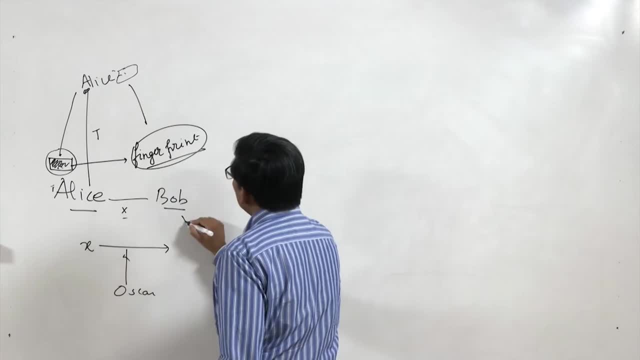 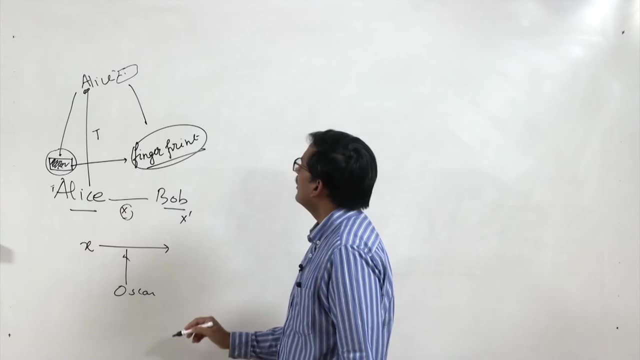 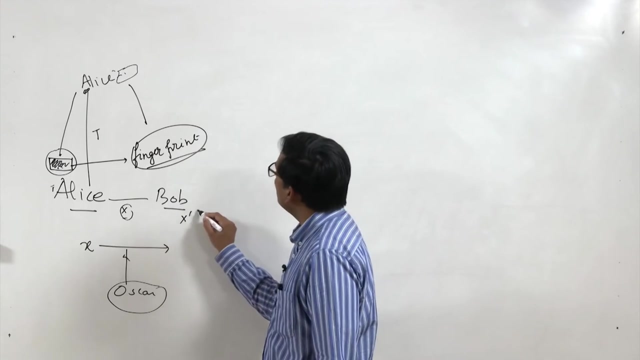 he gets something else in principle other than x. this x prime that Bob gets might be x itself, or the attacker Oscar might be interfering with this message and might have changed the message. So Bob definitely would like to know whether the message that he has obtained. 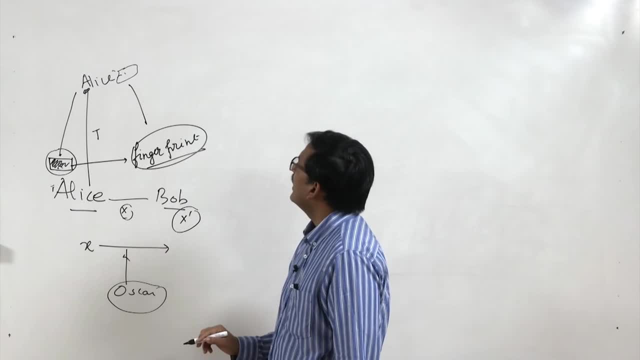 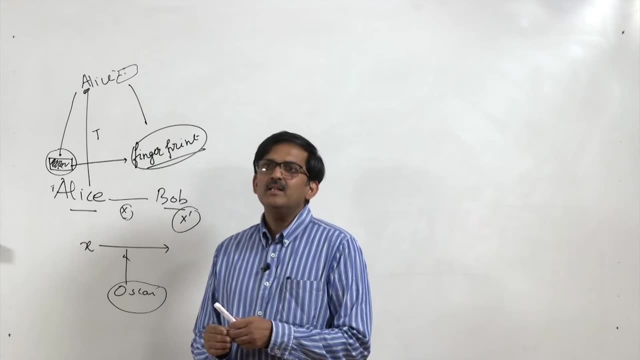 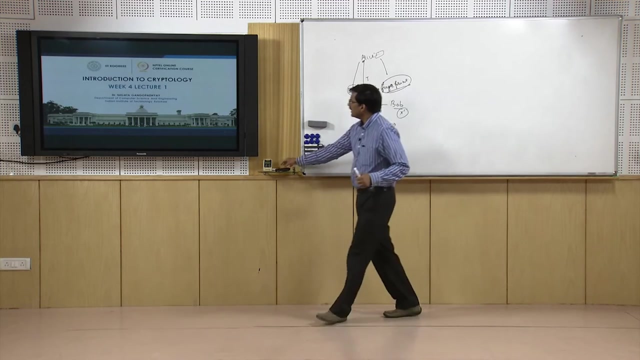 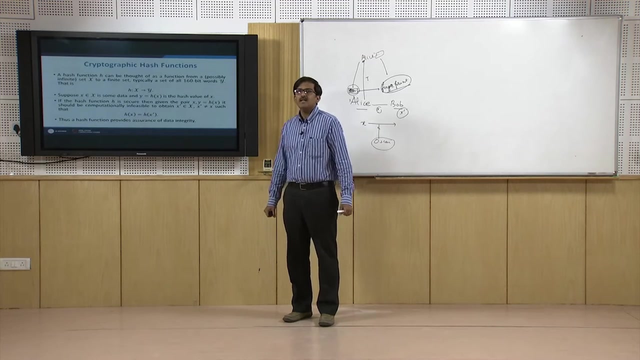 from Alice has been tampered with or not, And in some way, he would like to know whether, whether the message that is allegedly sent by Alice is really sent by Alice. So we start the topic of this week's lecture, which addresses these questions. 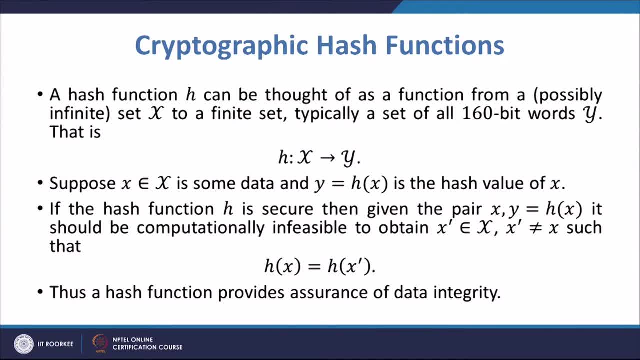 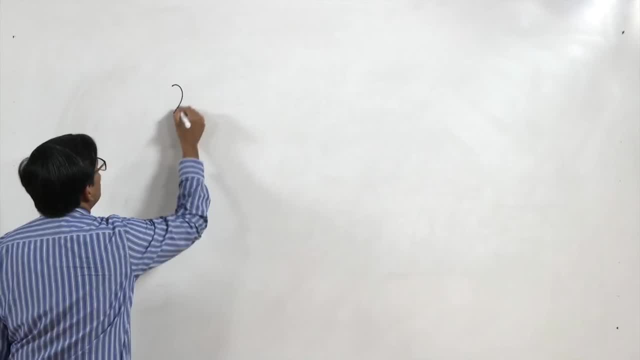 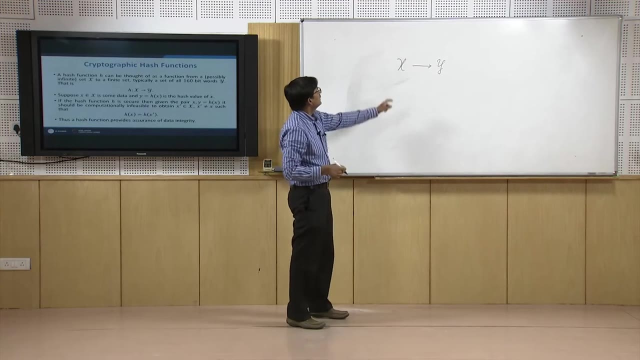 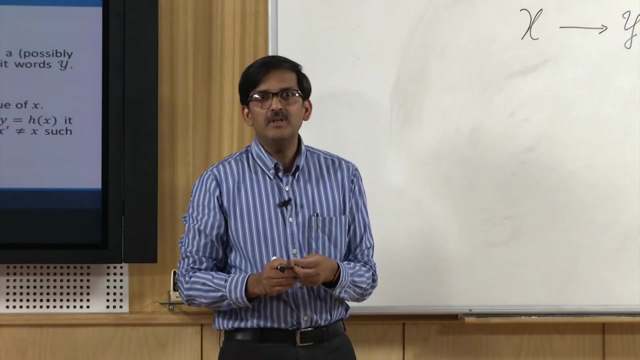 So we introduce cryptographic hash functions. A cryptographic hash function technically is a function from a space- let us say x- to another space, let us say y, such that x is very large, possibly infinite. y is relatively small. We would like to see how small is possible, keeping the security. 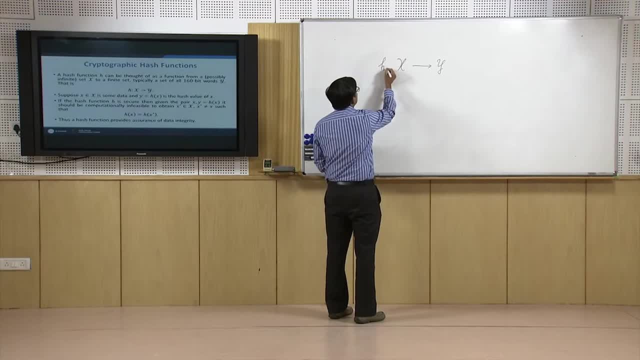 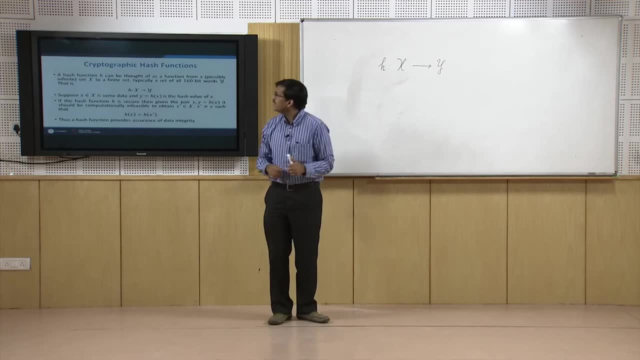 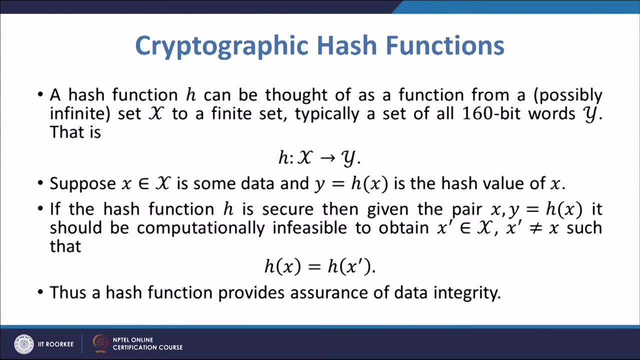 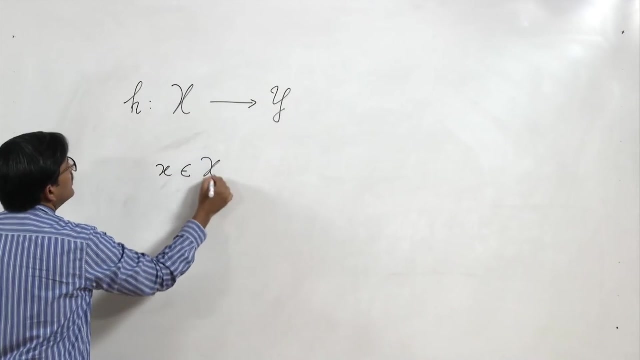 intact. So we will be denoting hash functions by h. So this is a hash function x to y and we have got certain names over here. very often, instead of message we will call elements of x as data, because in reality very often 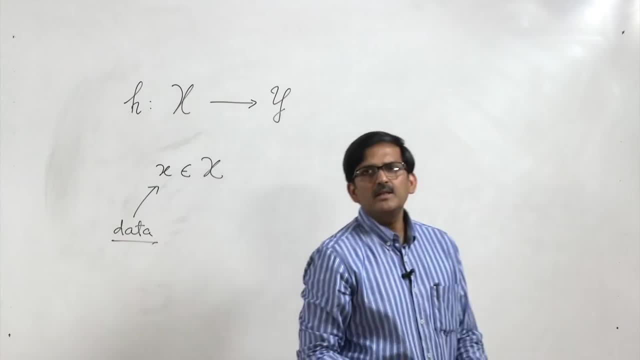 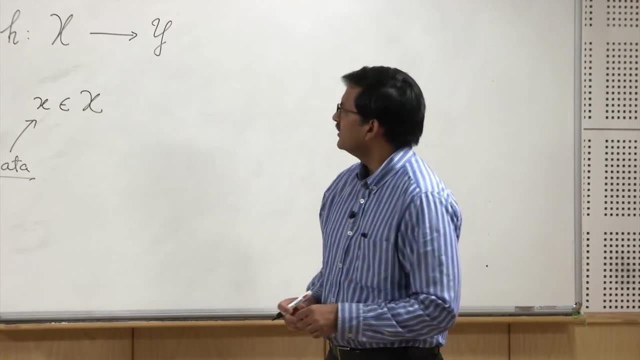 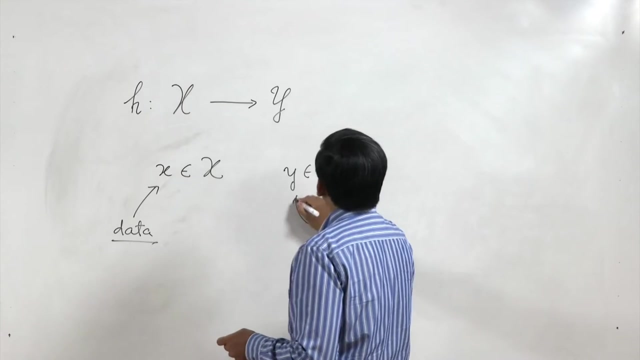 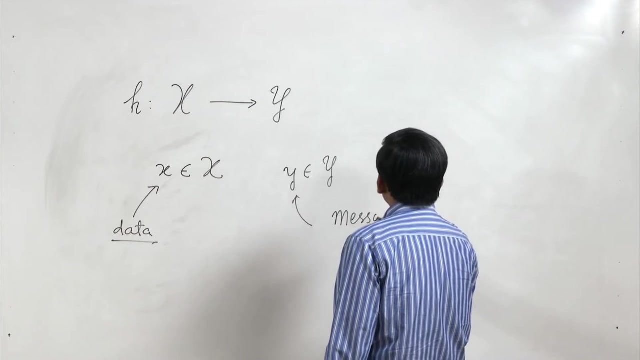 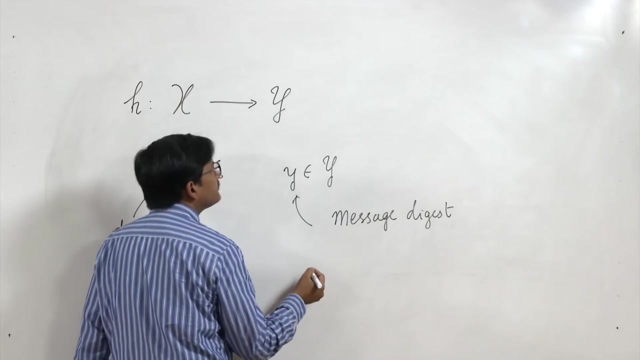 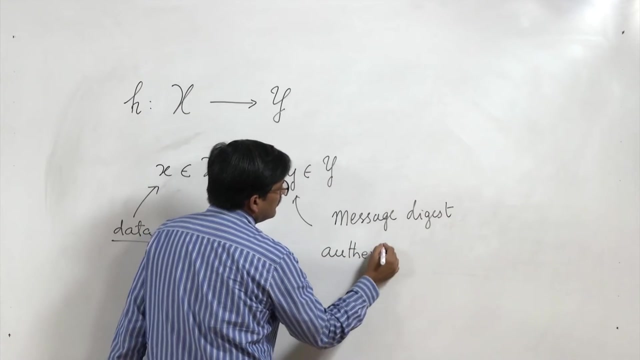 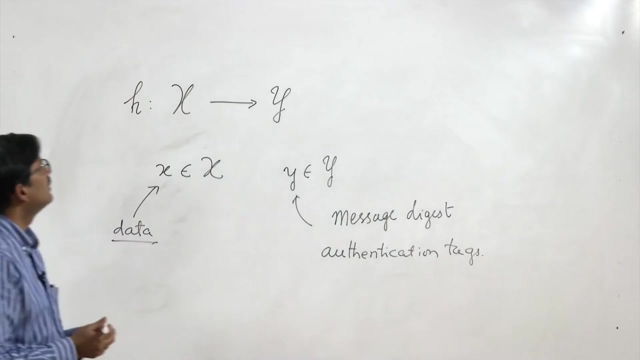 they will be data like, as I have been saying, that it might be a whole hard disk of Alice which she is leaving behind. So that is data and the elements of y will be called as data, So message digests or authentication tags sometimes. 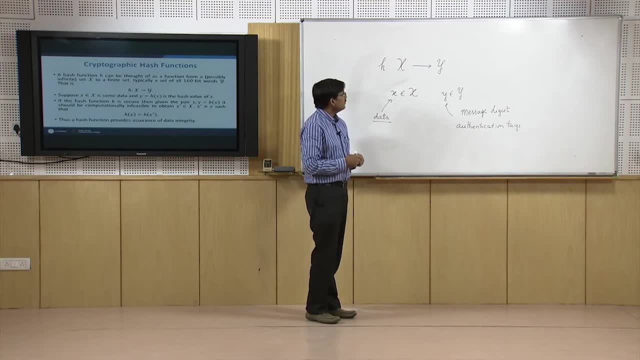 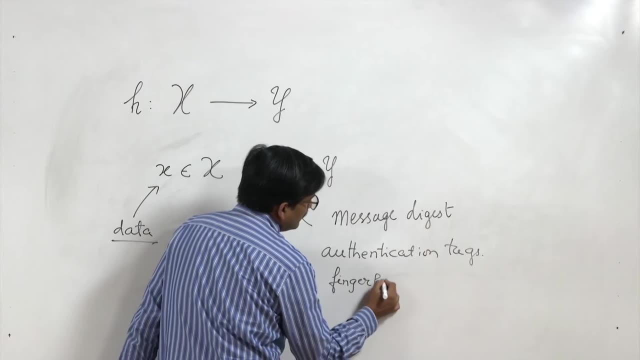 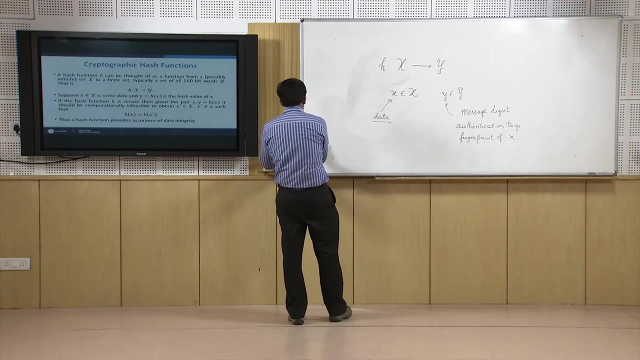 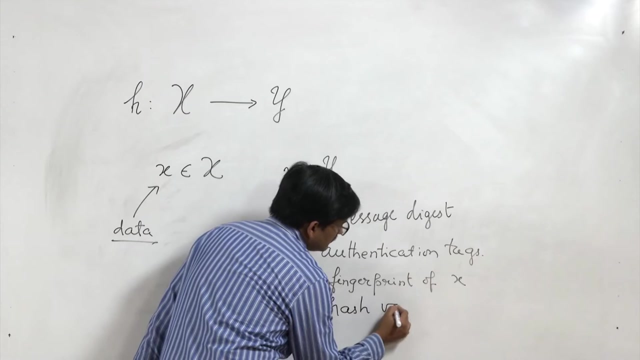 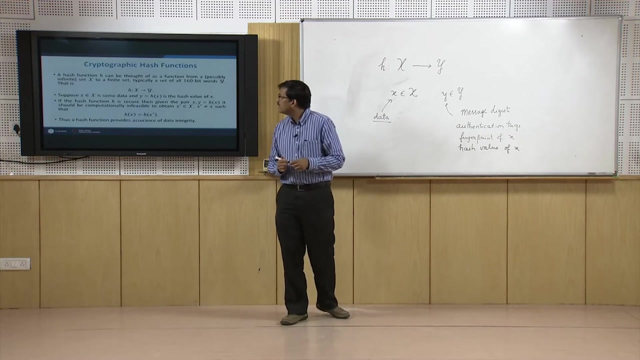 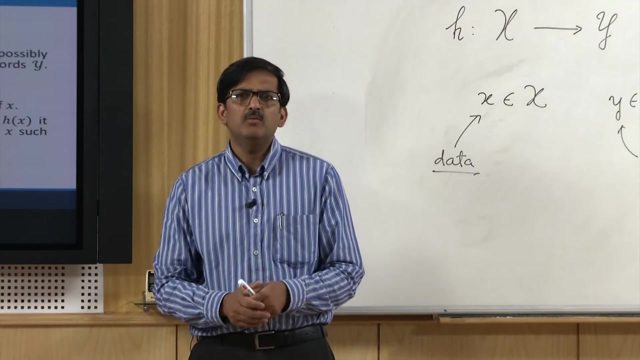 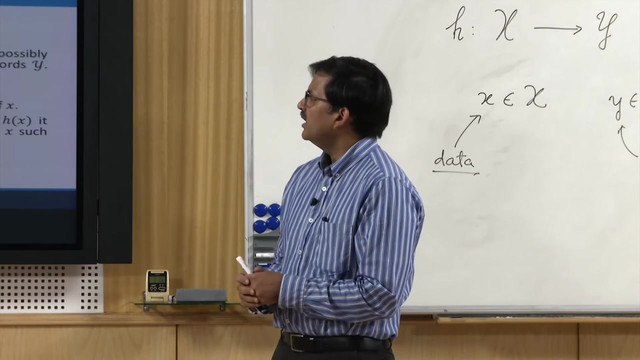 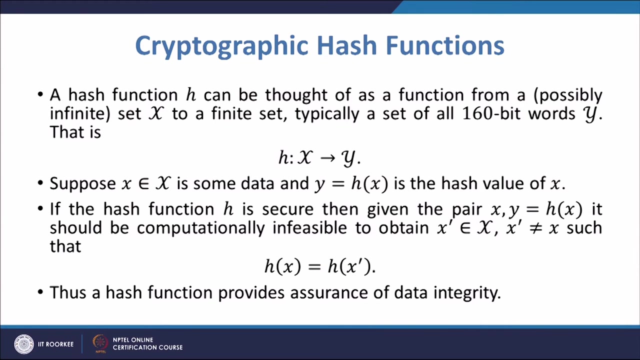 we may be referring to y as fingerprint of x or hash value of x. Now some basic level of security, what we want in a hash function. So let us look at this: If the hash function h is secure, then given the pair x and y equal to h of x, it. 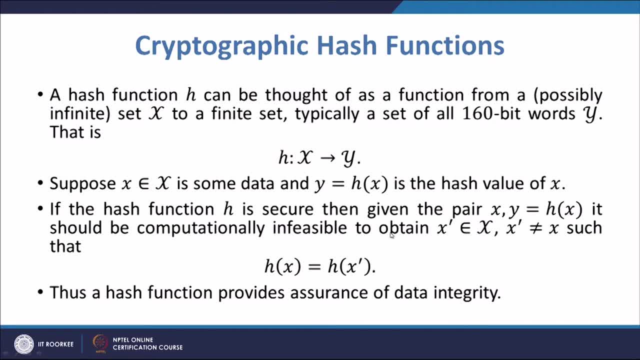 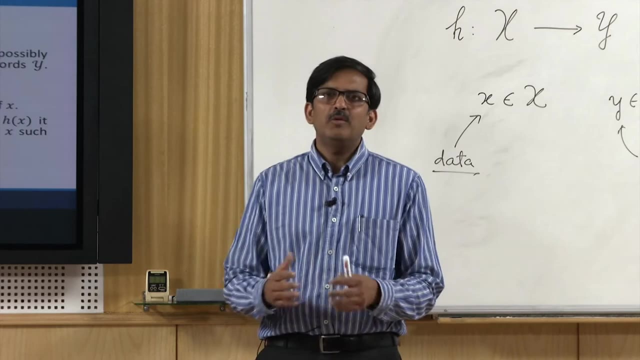 should be computationally infeasible to obtain the hash function Another data x prime belonging to x, such that x prime is not equal to x and h x is equal to h x prime. So this is how we will get some kind of data integrity. So what will? 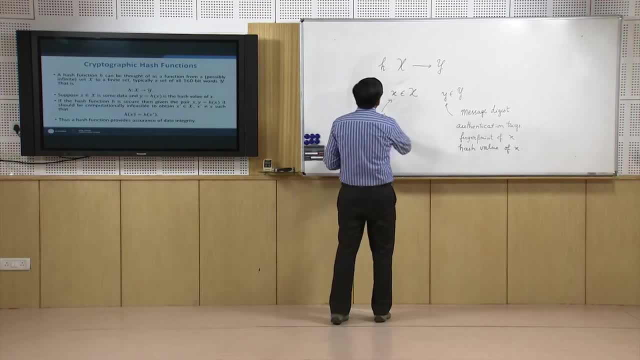 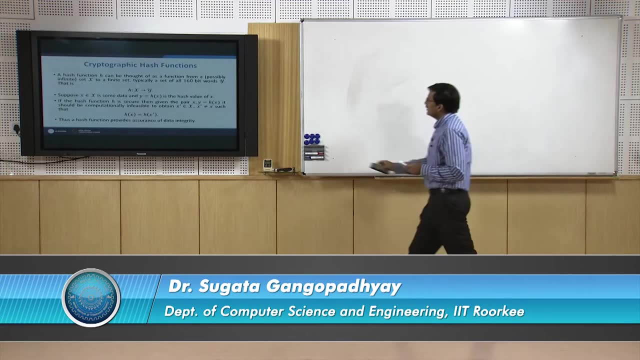 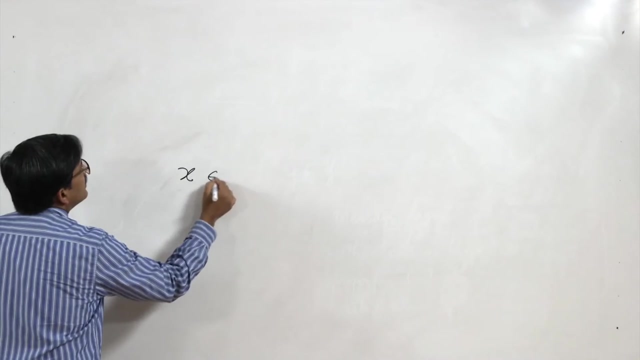 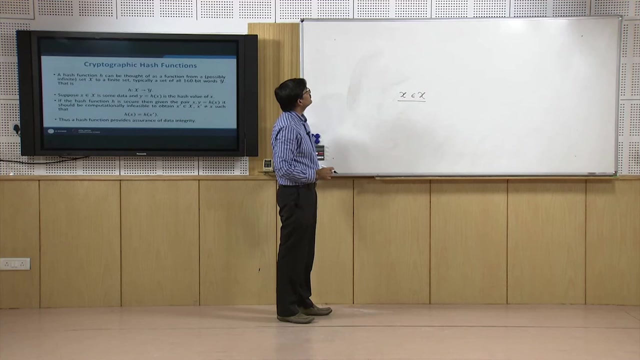 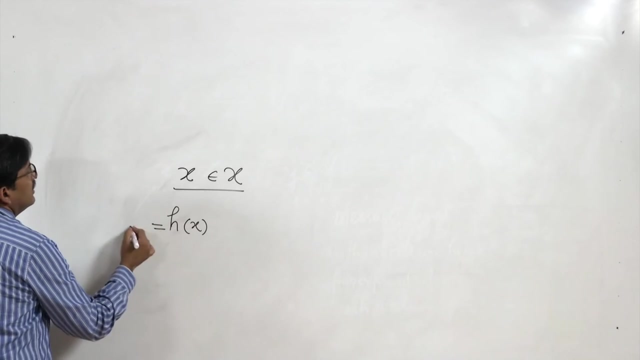 happen for Alice. If Alice has access to a hash function, the data in a hard disk x which she wants to protect is she will apply the hash function. hash function h on x and get y. this y is small, much smaller than x, and she will carry. 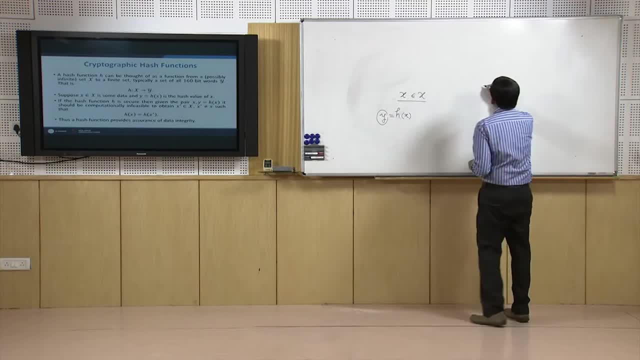 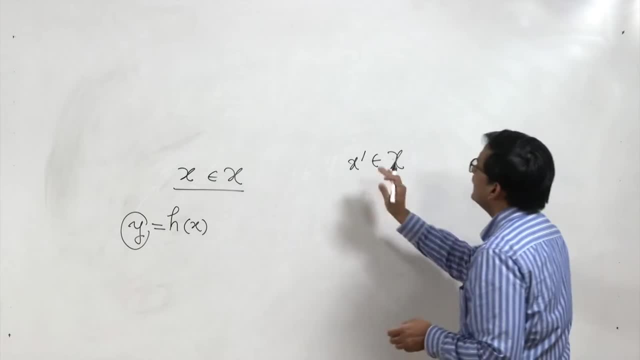 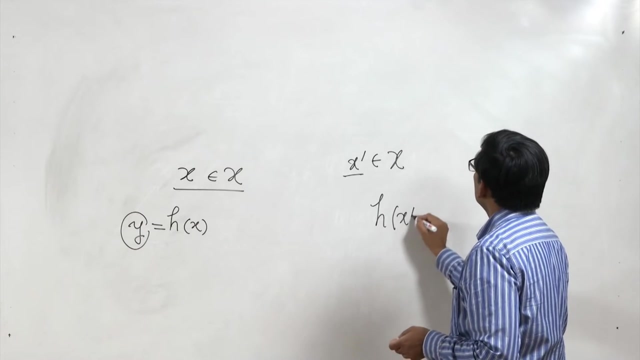 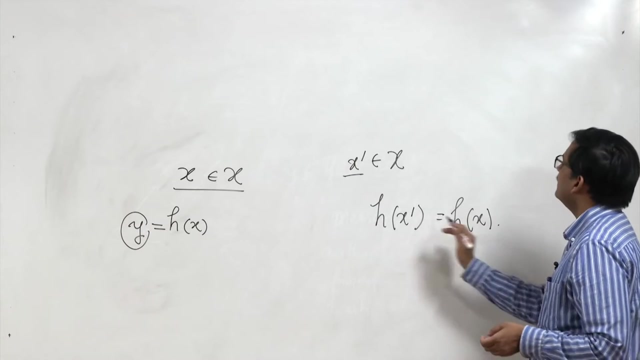 the y and when she comes back she has got she will look at the look at her hard disk that she has left with the data. So data is x prime and then she will compute h x prime and she will match h x and h x prime. If she finds that both are same, then with high reliability. 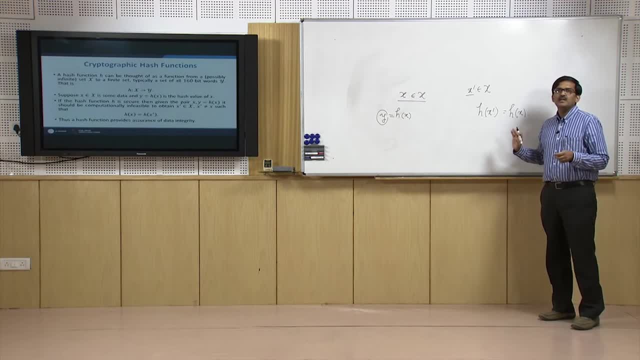 she will infer that no one has tampered with her data. but if they are not same, then she will definitely be able to say that someone has tampered the data and So therefore it will be very- it must be very, very difficult to find out the data. 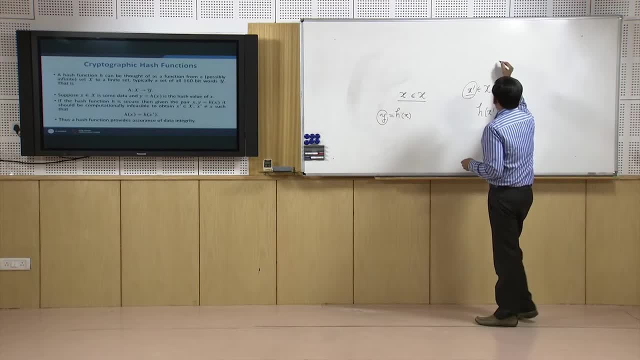 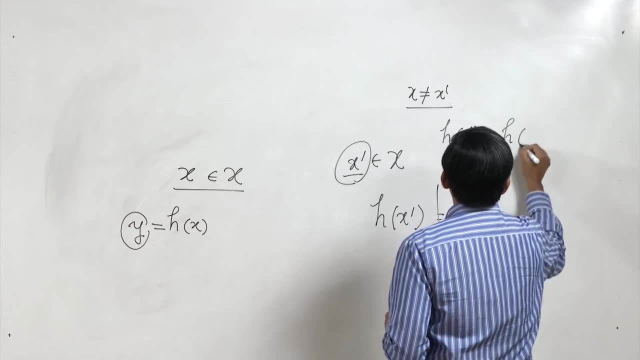 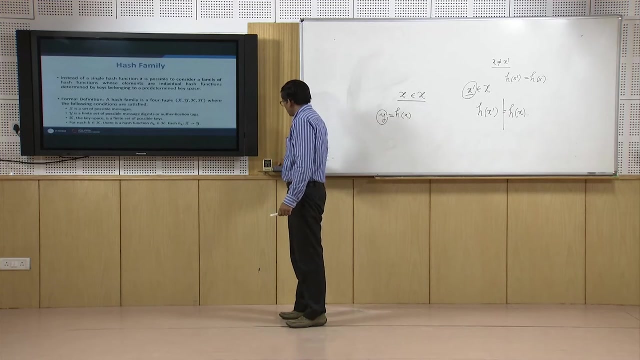 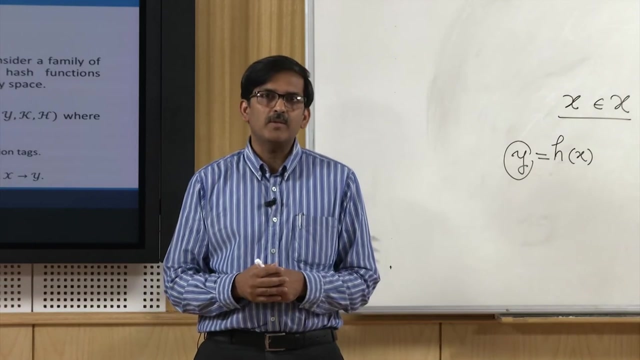 So find out an x prime such that x is not equal to x prime, but h x prime is equal to x. Now we can move on to something more general, from hash functions to hash families. What we can do is that we can create a kernel of 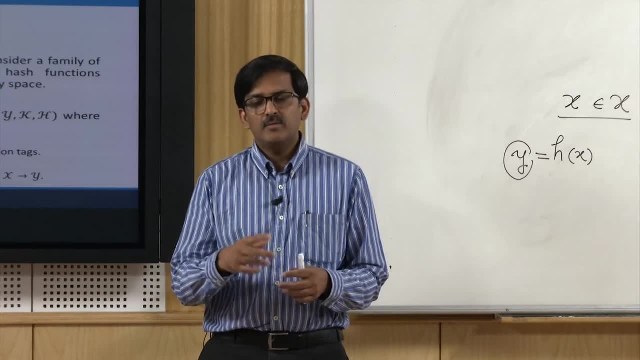 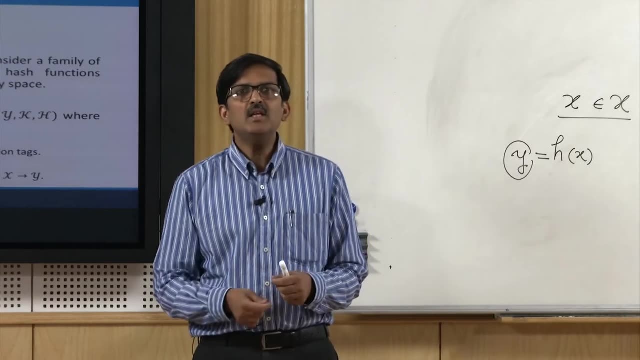 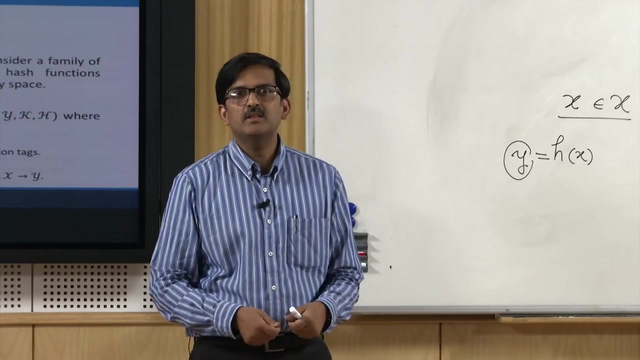 a class of functions which are dependent on a key, So that whole class will be called an hash family and the key is like our usual cryptographic keys, which will be exchanged between Alice and Bob and a particular hash function from the family will be will be obtained. 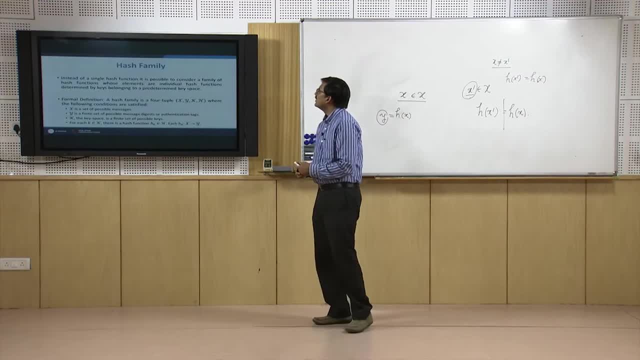 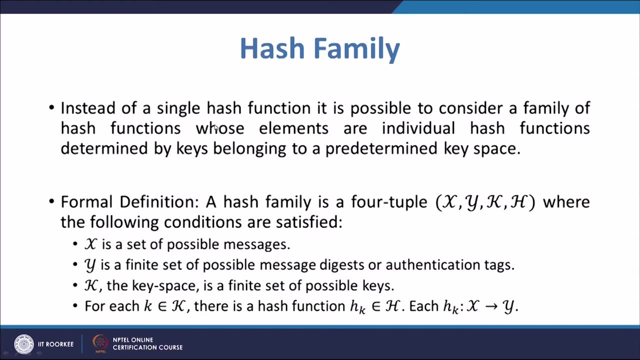 by them. So let us see, instead of a single hash function, it is possible. So let us see, instead of a single hash function, it is possible to consider a family of hash functions whose elements are individual hash functions determined by keys belonging to a predetermined key space. Now, formally, we will define a hash family. 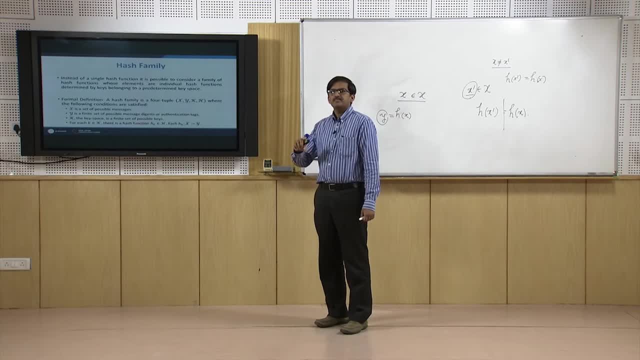 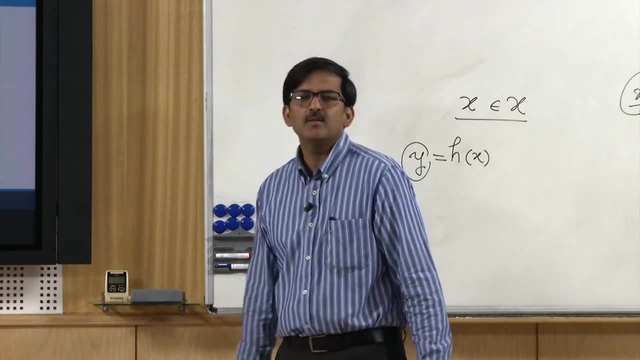 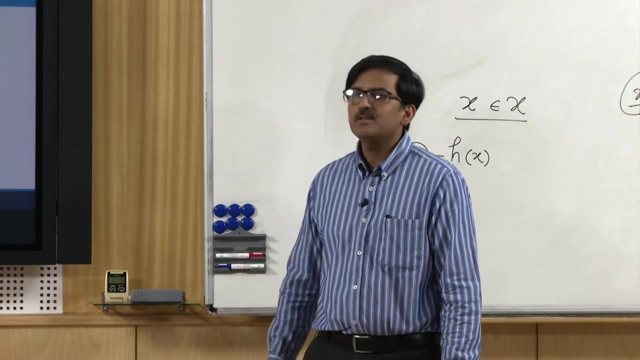 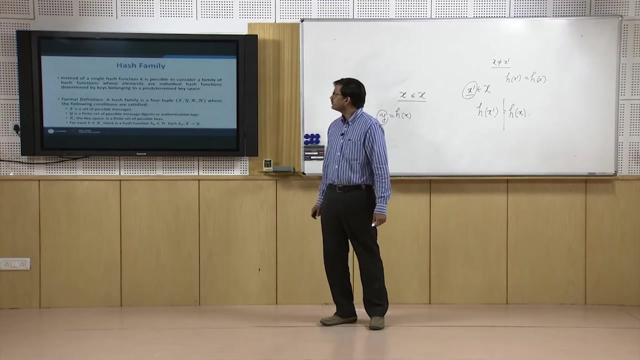 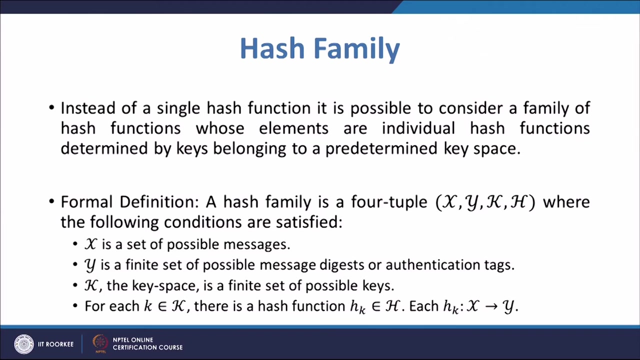 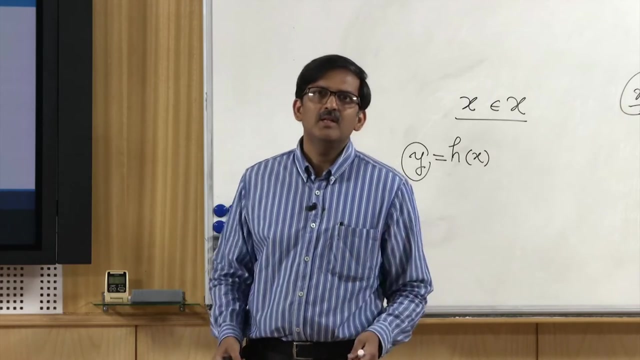 as a four tuple. So we will have a space of data, that is x, then we will have a space of message digest or authentication, Authentication tags, which is y, and we have a space of key and a family of functions. So, given a key K belonging to capital K, Alice and Bob will be able to obtain a function. 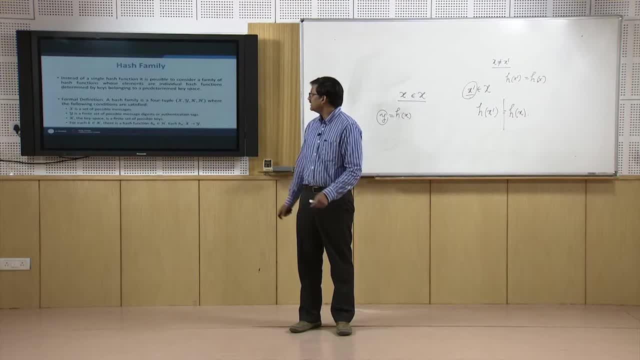 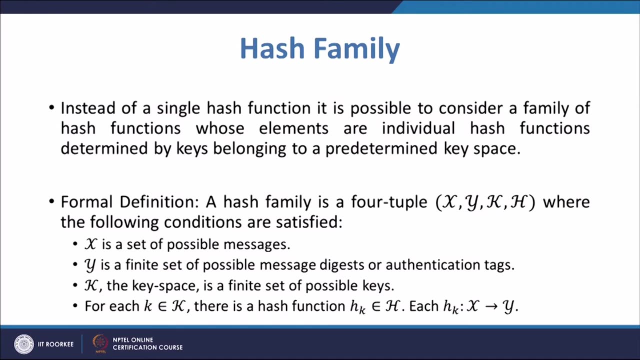 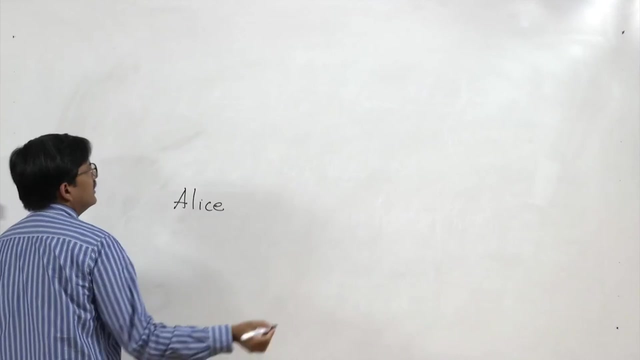 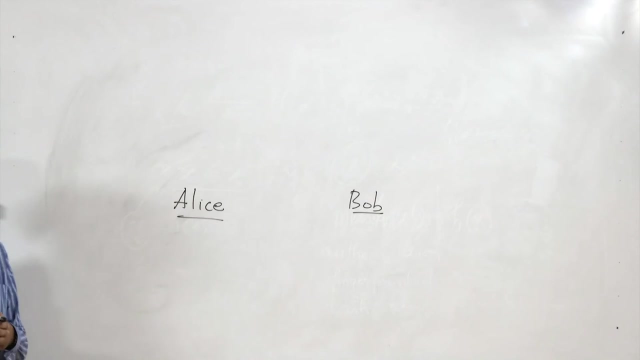 in H, which they they will denote as a key H sub k and which will work for their requirements. Now it might be like this: suppose Alice and Bob are communicating. Now what Bob and Alice wants to ensure is that when they are, 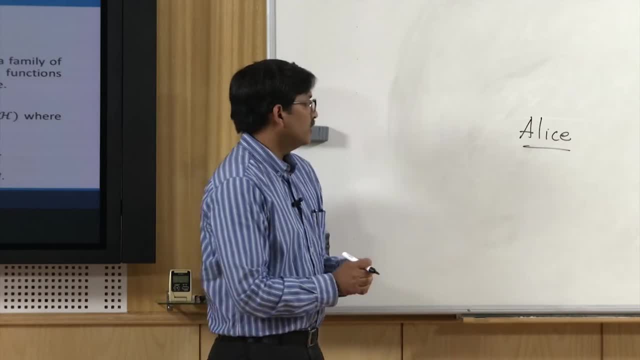 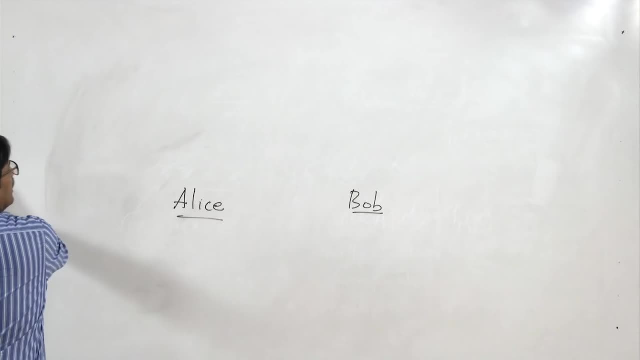 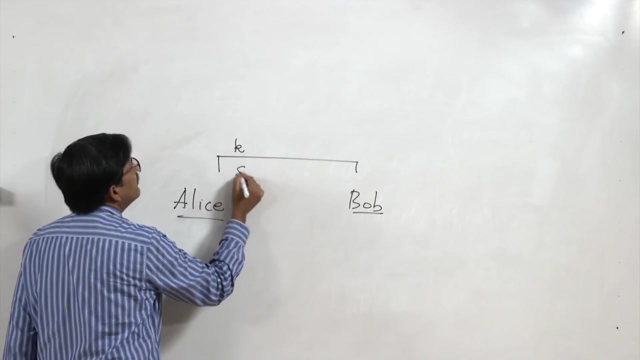 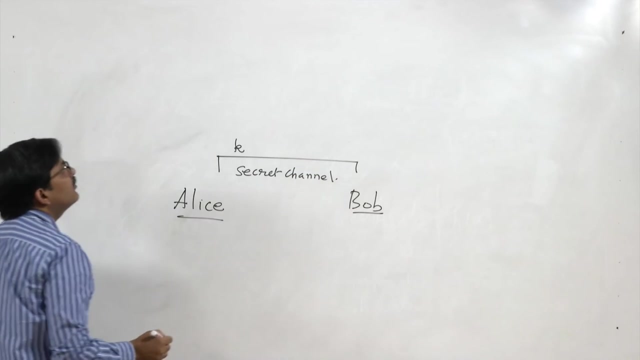 sending the message. nobody is tampering with it. So what Alice does is that Alice takes the data first. what they do is that they agree up on a key through a secret channel. now this has to be done by a, through a secret channel, and since they are agreed upon a. 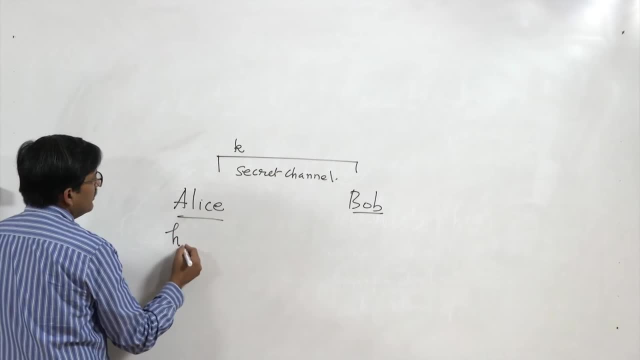 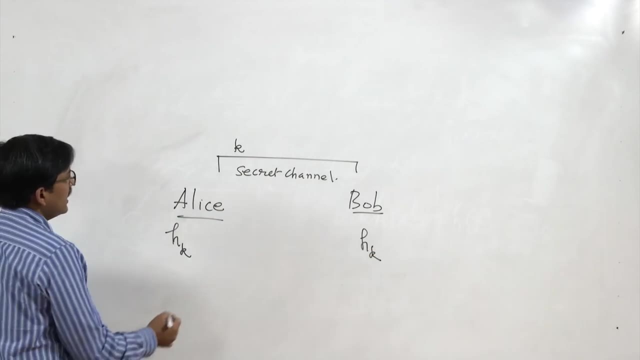 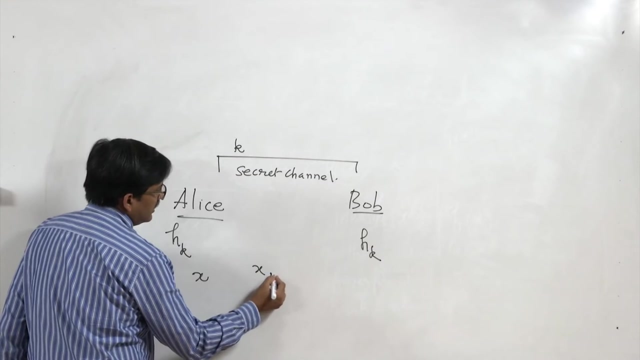 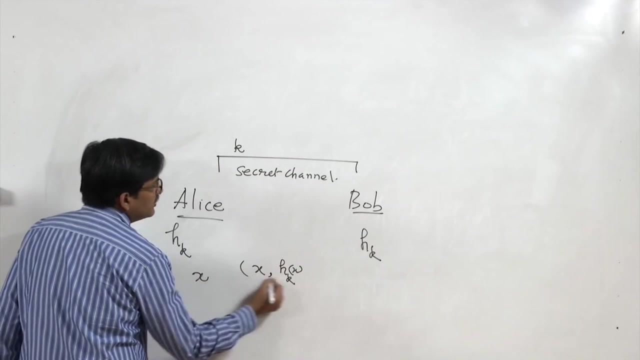 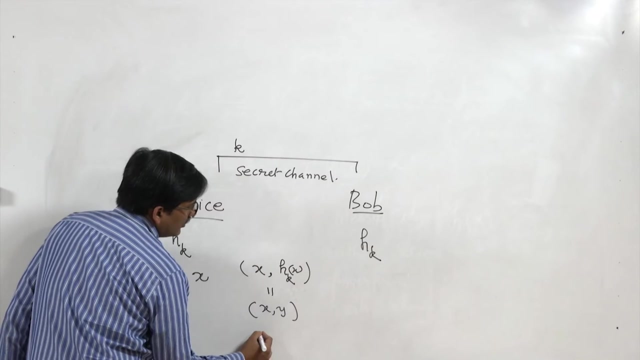 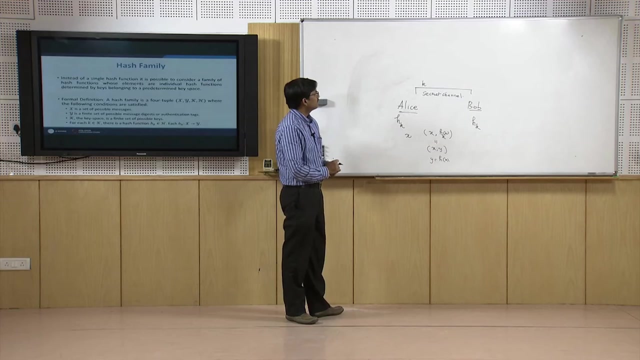 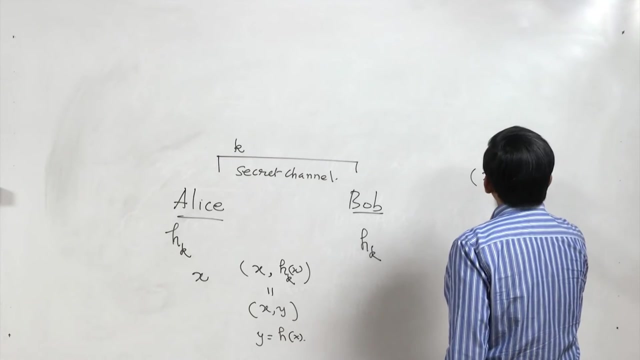 key. both of them will have the hash function h sub k. Alice wants to send x to Bob. she sends a pair. she sends x and h sub k, x, this pair, which we will denote by x, y, where y equal to h x. Now Bob obtains this pair. and now 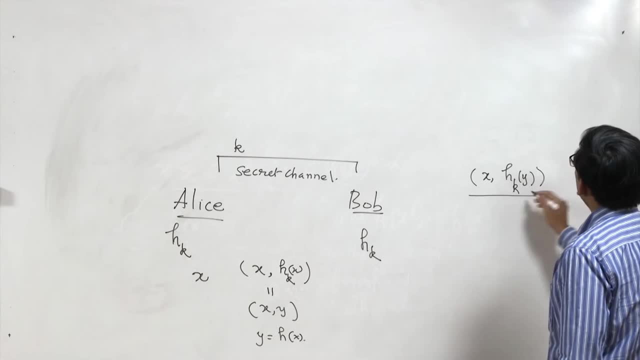 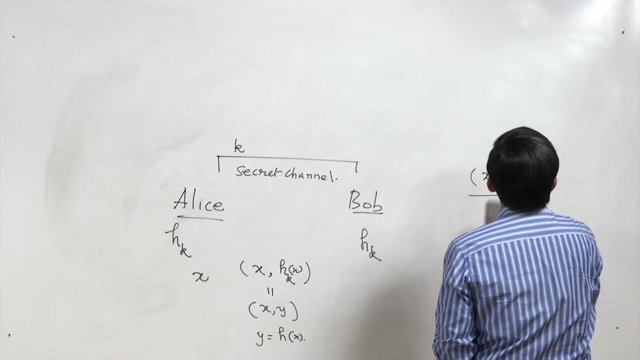 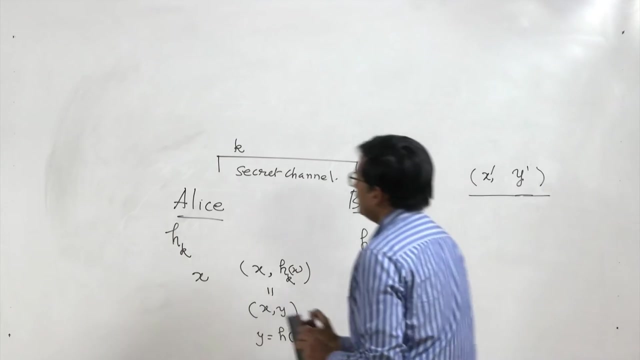 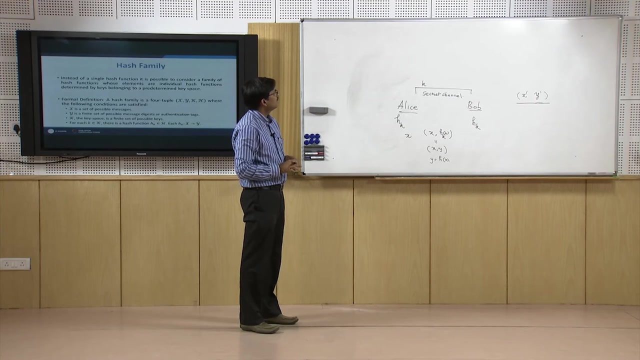 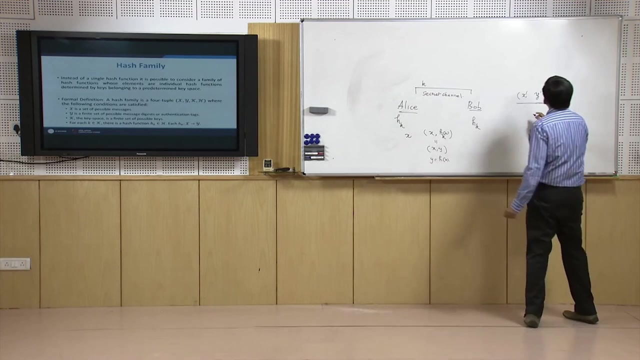 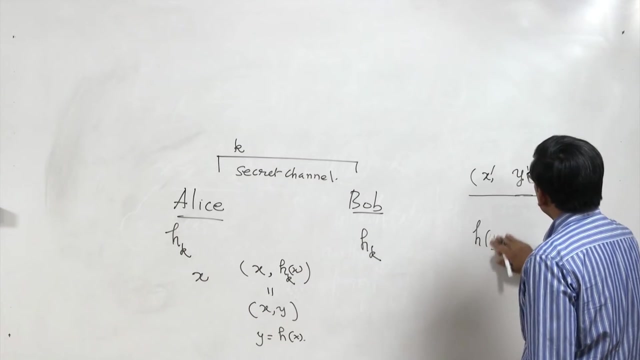 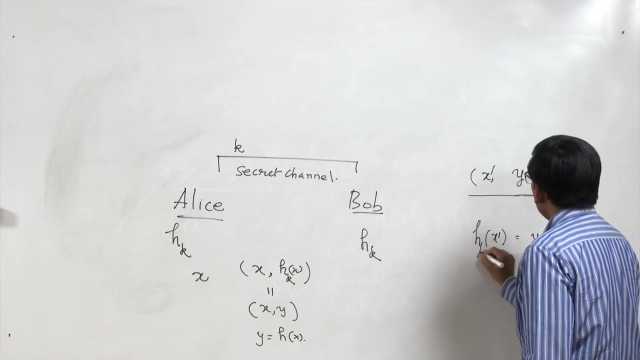 in reality, Bob is not sure Whether he has obtained this pair or a modification of this, so that is why we are writing that Bob has obtained this and this is not h k y. this is y. Bob has obtained this. So what Bob does is that Bob computes h x prime and checks whether it is equal h k x. 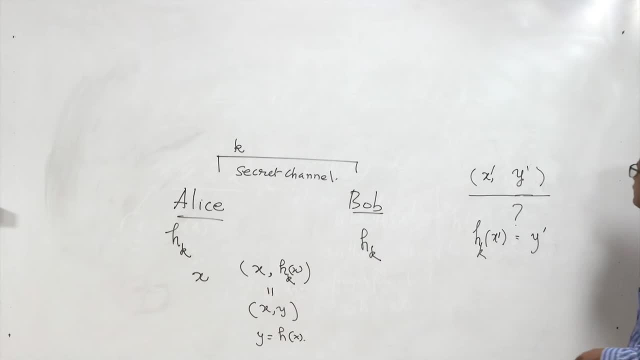 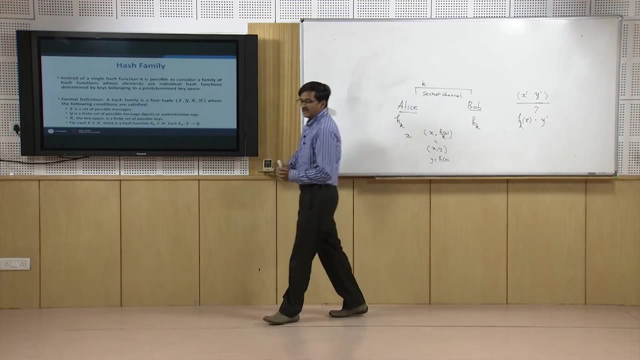 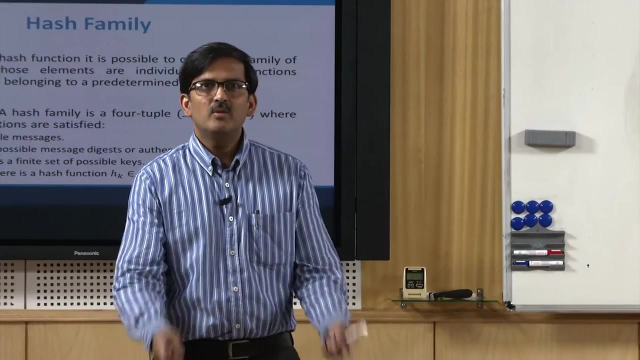 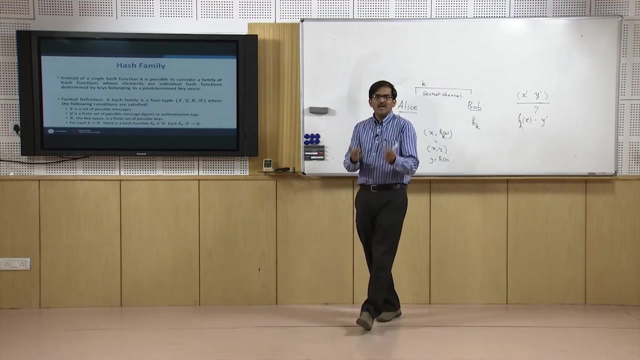 prime, whether it checks that, whether it is equal to this, What this hash function must guarantee me. So if I do not know the key, it will be computationally infeasible to find out a pair which is valid for this particular function. So an attacker cannot produce a pair like this: x, prime, y. 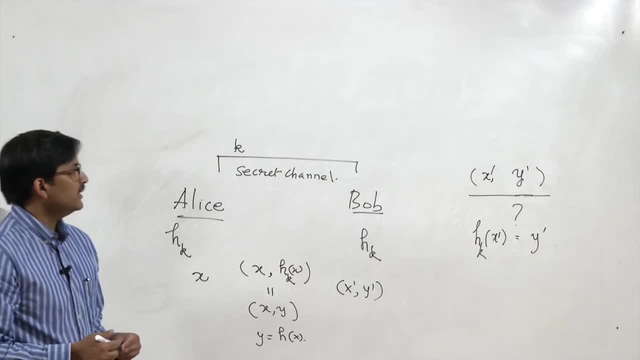 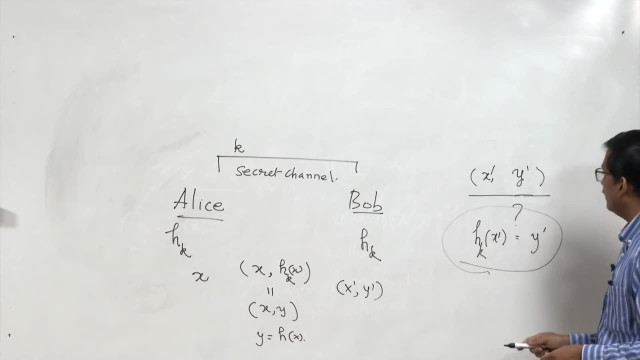 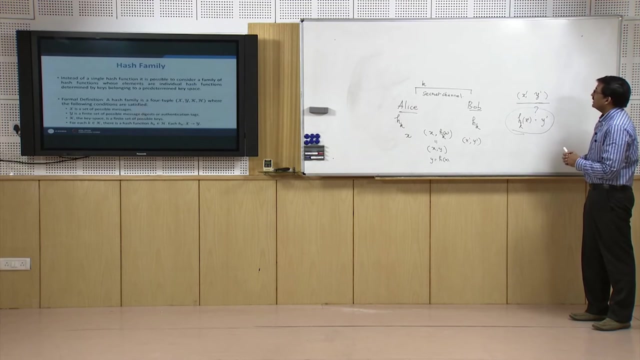 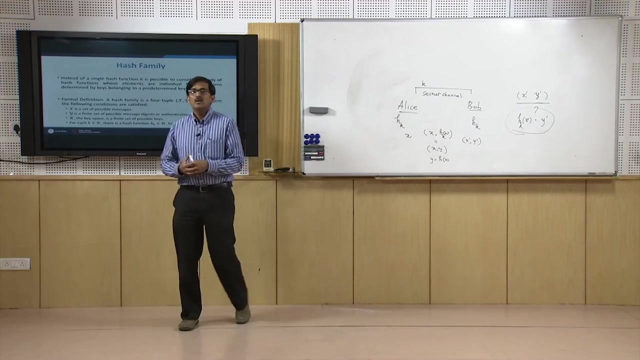 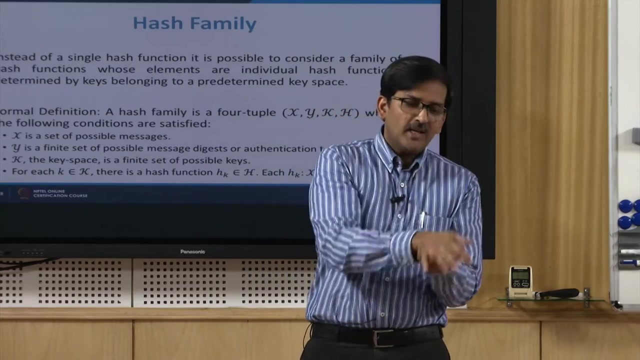 prime and send to Bob, take it out, So that Bob, when checks with this equation, will find that this equality holds. So if such is the case, then Alice and Bob has obtained some authentication. So if, whatever Bob gets, Bob applies hash function that particular. 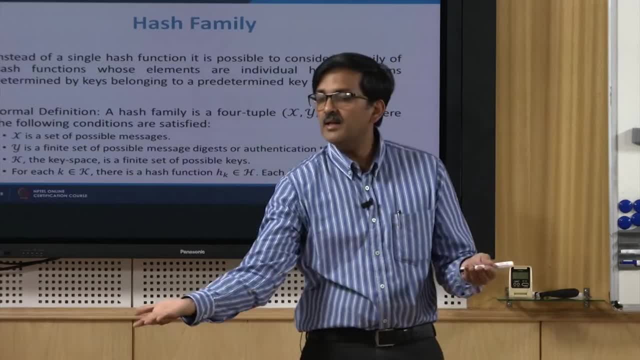 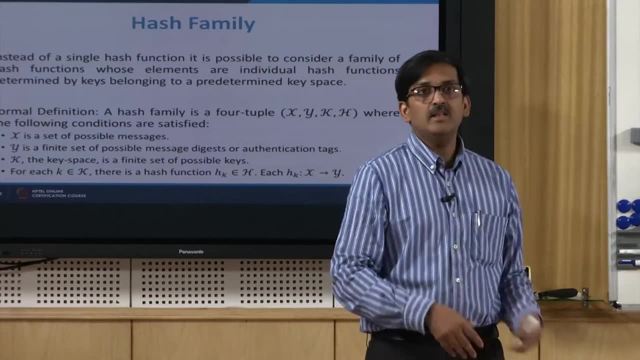 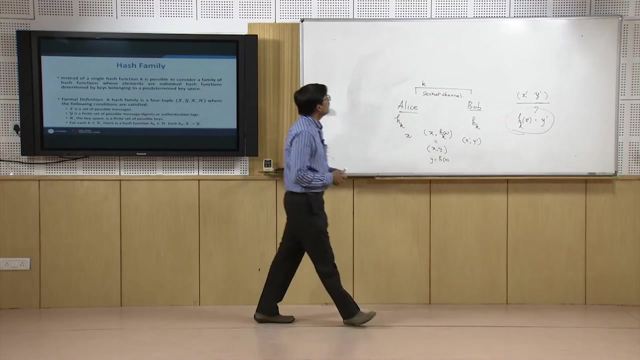 keyed hash function to the message and checks the message digest. If they agree, then Bob should be quite certain that the message is all sent by Alice and no one else, and Alice as message has not been tampered with. So that is what you would like to achieve. 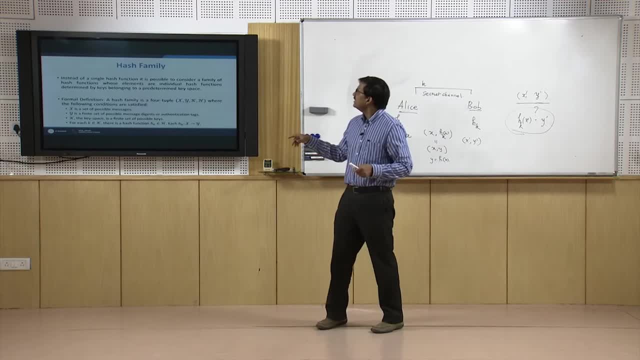 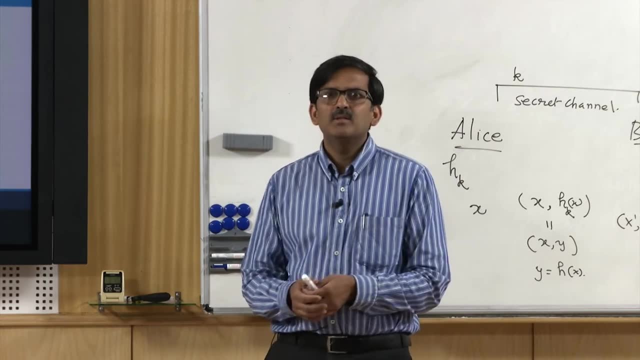 What we see is that unkeyed hash functions are also, in a sense, fall within the same same property of some sketch function, So these could be called as hyperboles, but we are not having any singularities there. Of course. we have a still of the, the inequality, where 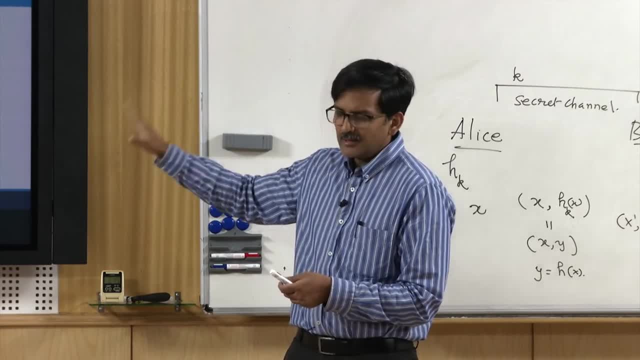 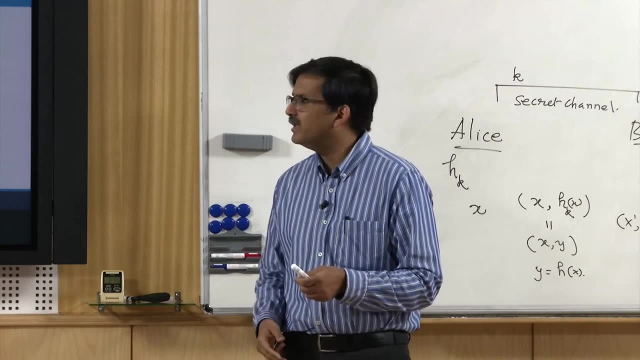 provides a simple law or, de facto, the property of missed hash reason, as I have shown in the Dolby mac weird conservation. Well, what we want to highlight also and what is guaranteed same framework. we can always say that an unkeyed hash function comes from a hash family. 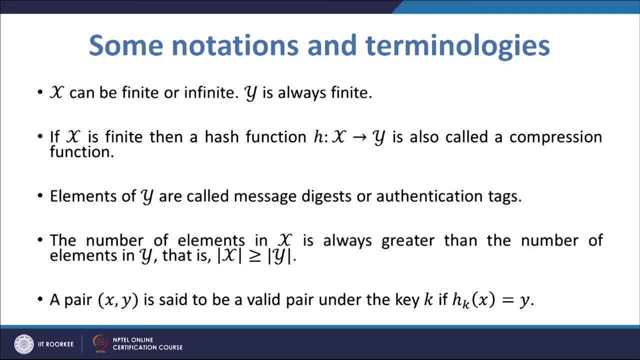 where the key space is singleton. Now let us come to some notations and terminologies. alright, So, as we have already seen that the set of data x can be finite or infinite at, y is always finite and relatively small, then if x is finite, then the family, then the 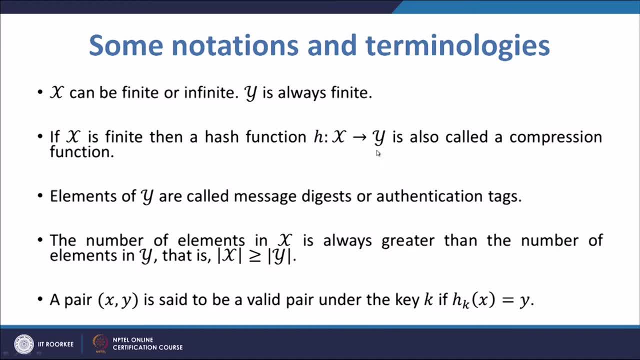 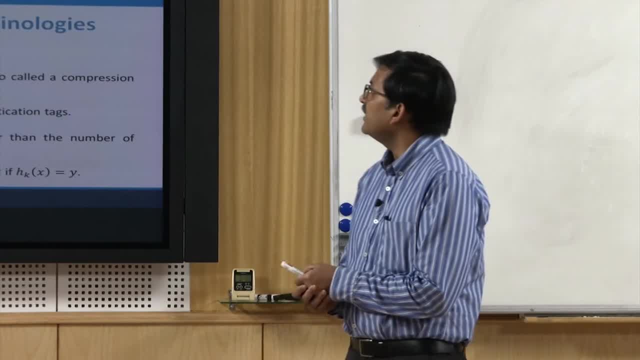 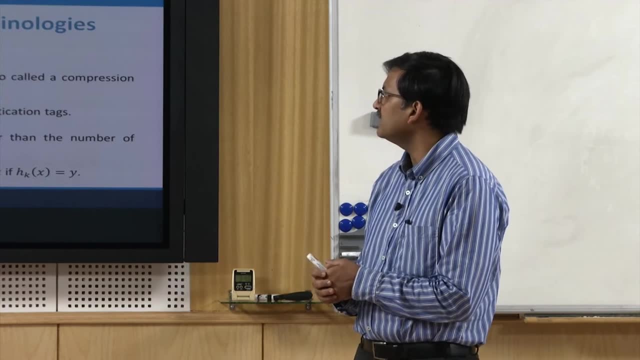 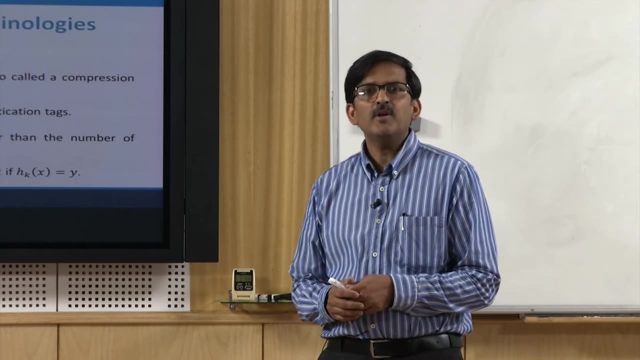 function h from x to y is also called a compression function. We will be using this terminology very often later and we have already said that y is a is. the elements of y are called message digest or authentication tags, And the number of, even if x is finite and the number of elements in x is much larger. 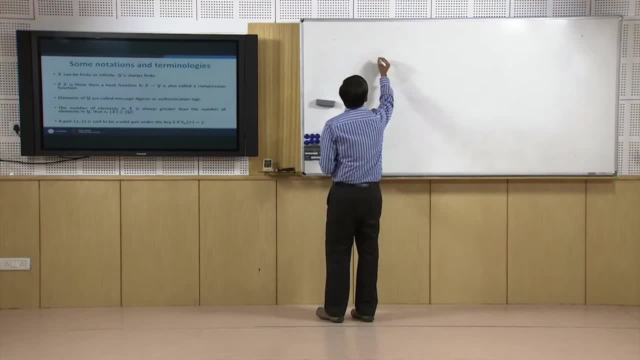 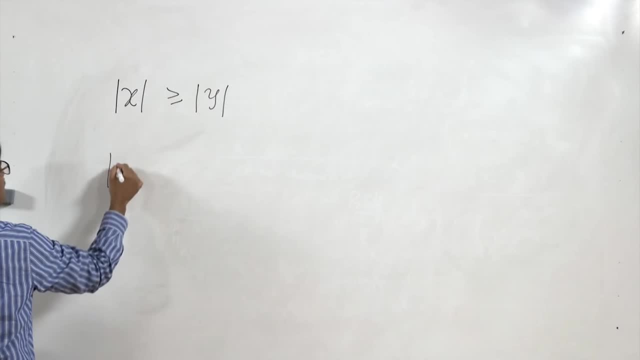 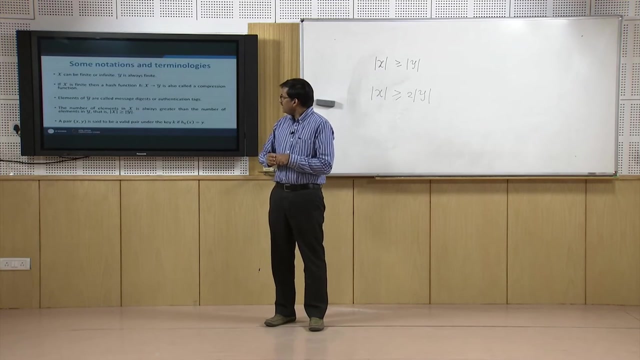 than number of elements in y. So, of course, we will have this relationship always. In fact, we will be having something else, something more stringent as this, that is, number of elements in x will be twice more than Twice the number of elements of y, and there is a concept of valid pair. If I give you 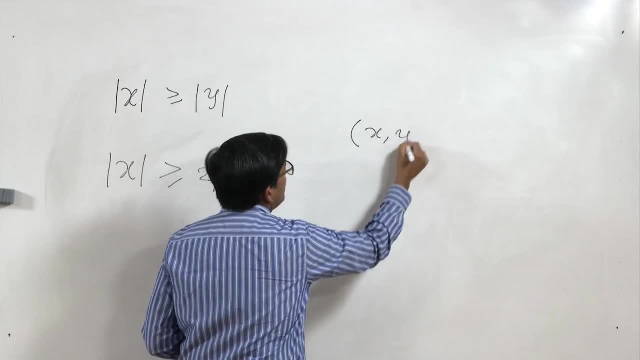 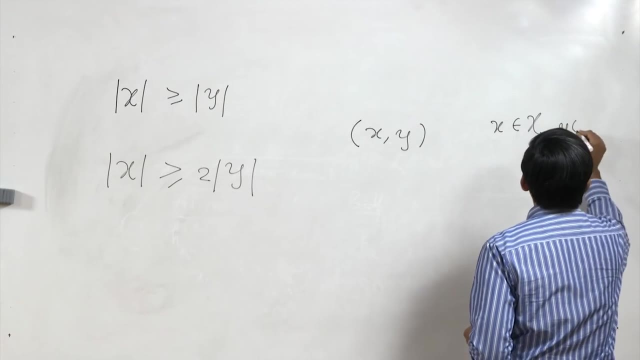 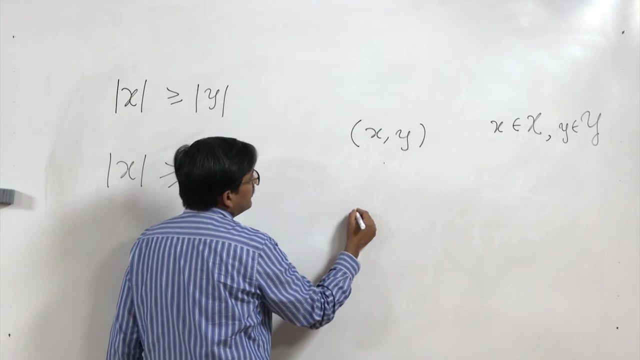 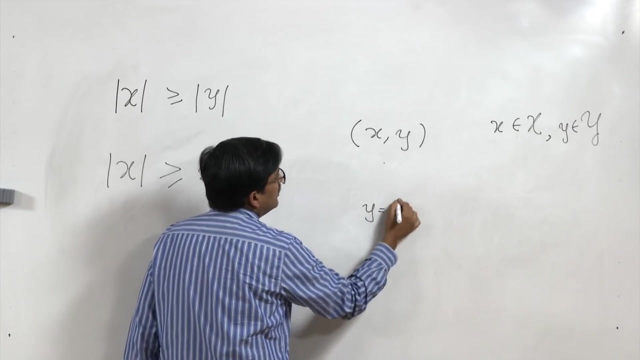 a pair x- y where x is an element of capital X and y is an element of capital Y, then we will say that x- y is a valid pair if, and only if, y is equal to h- x. So this is also a terminology that is used very often. 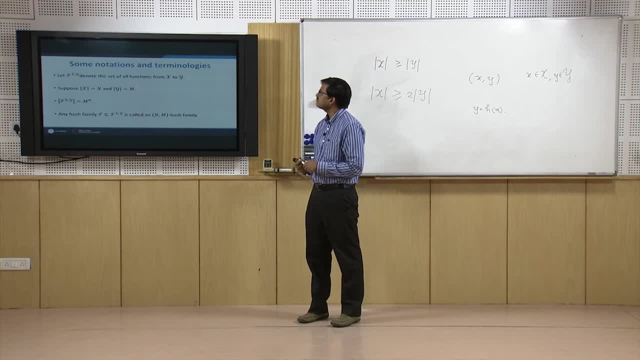 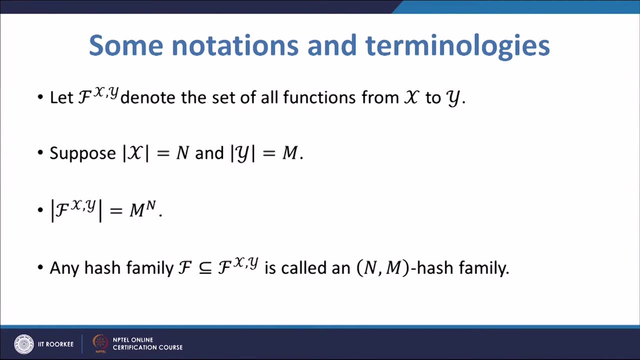 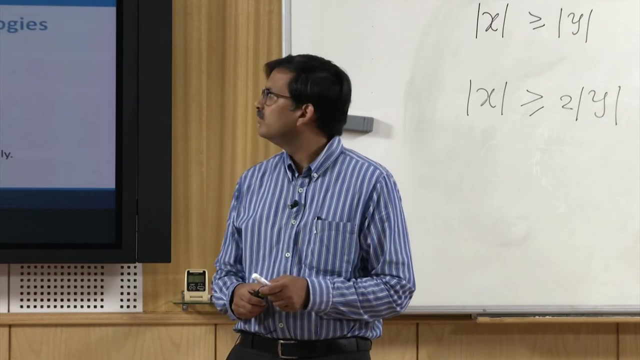 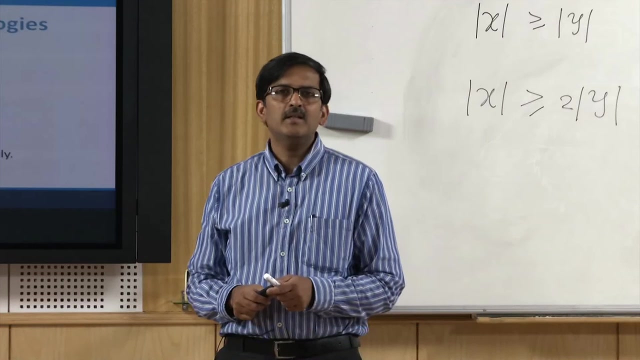 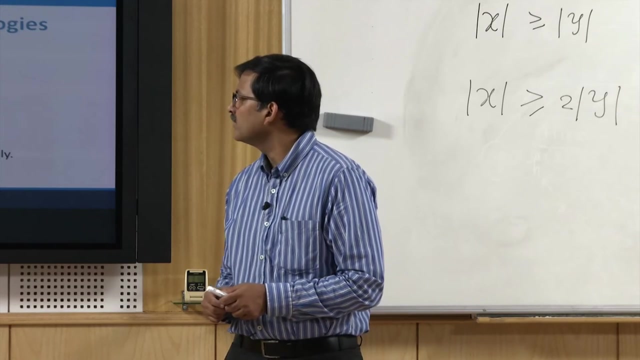 Now some more terminologies. by f, superscript, x, y we will denote the set of all functions from x to y, And very often the number of elements in x, if x is finite, will be denoted by capital n, and number of elements in y will be denoted by capital M And in that case the number 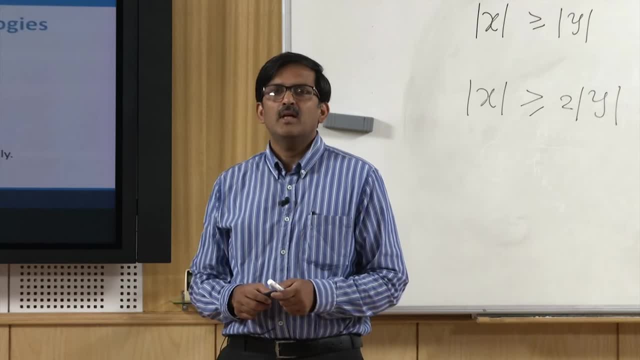 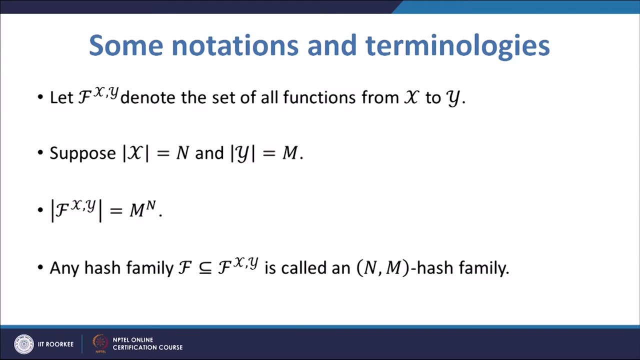 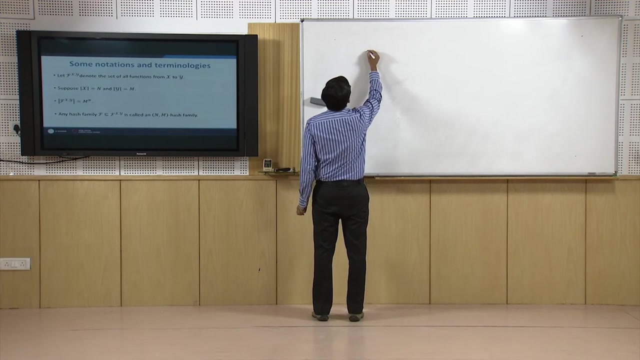 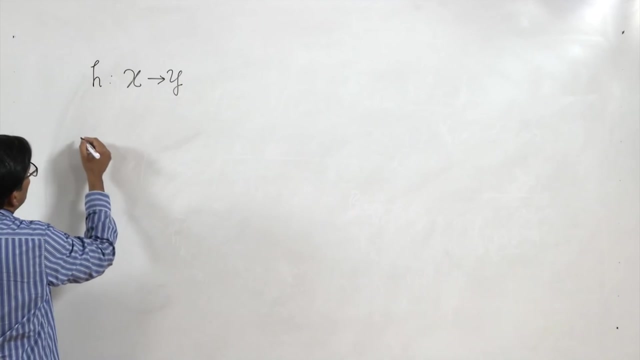 of functions in f superscript: x, comma, y will be M, raise to the power n. Let us quickly have a look at this counting. So we are considering all the functions from x to y and we are denoting that by f superscript. 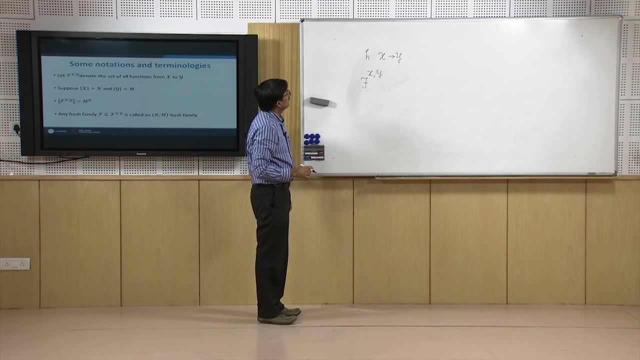 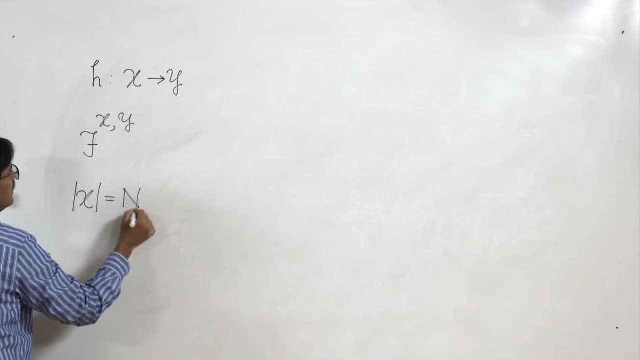 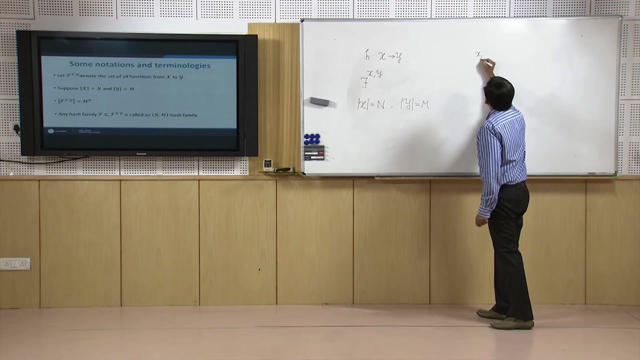 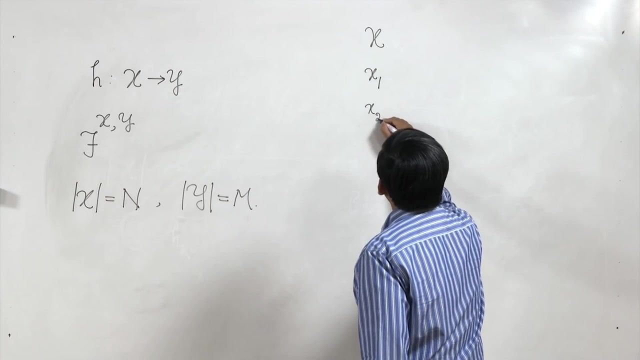 x, comma y And we have been told that the number of elements in capital X is n and the number of elements in capital Y. So if we list all the elements in script capital X, that is a domain, So we can list. 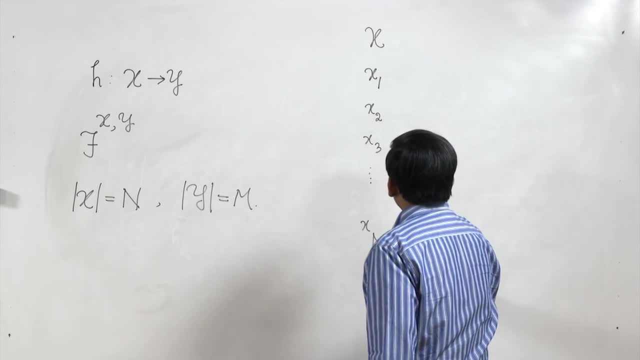 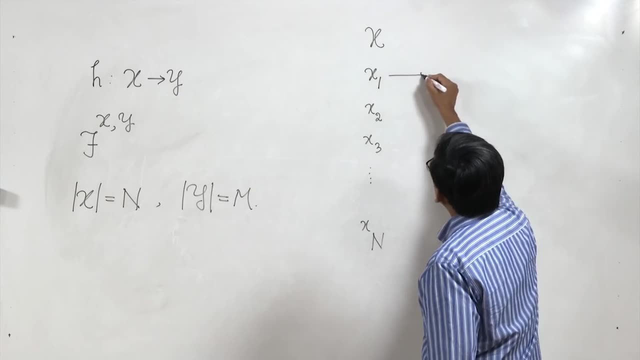 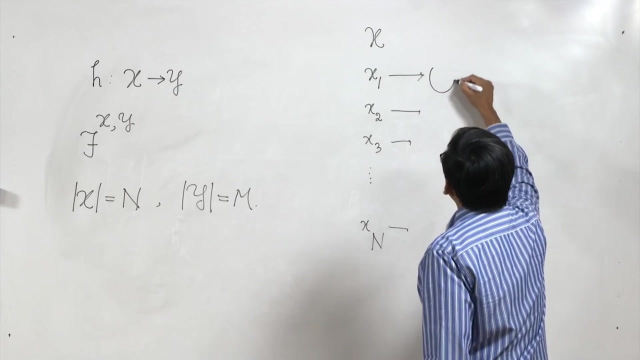 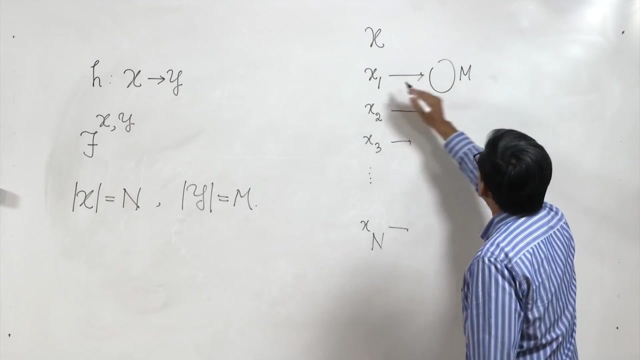 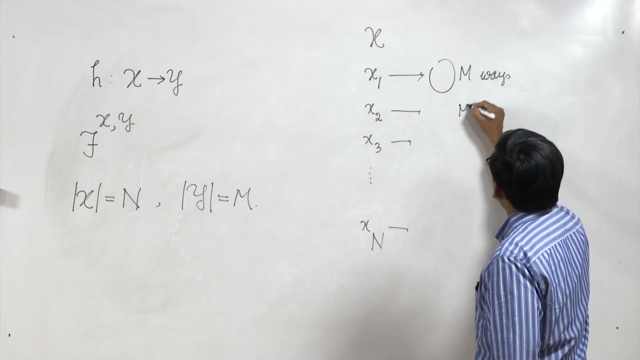 like this: We come up to x sub capital N And what we see is that we can choose the image of x i's, that is, x 1, x 2 and so on, in m ways. each of the images can be chosen in m ways And therefore the total number of choices is m into m into m. 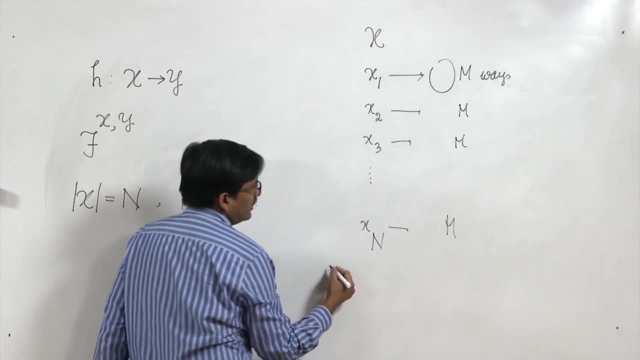 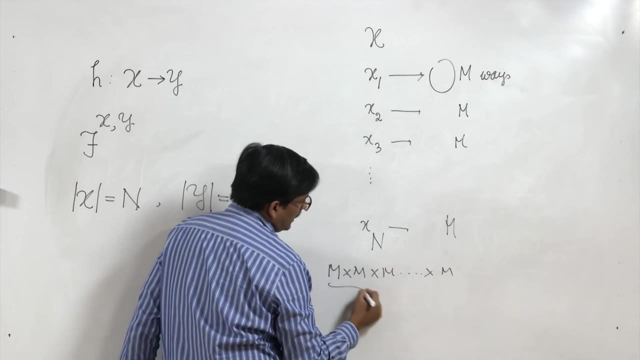 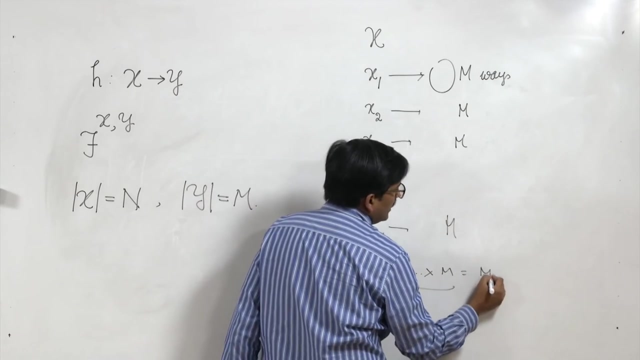 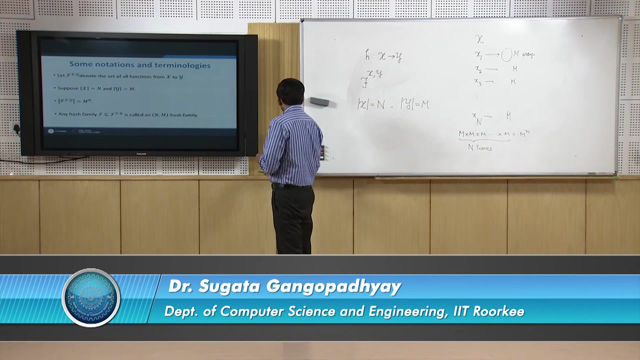 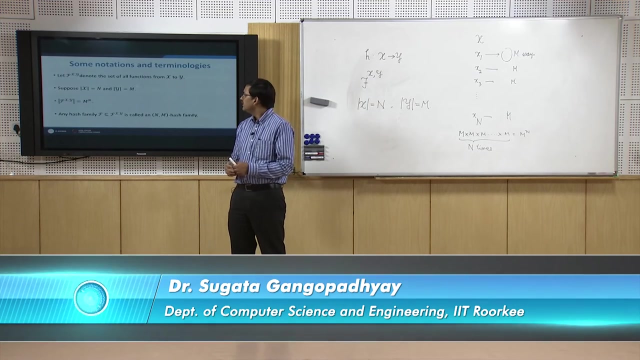 capital N times. m into m into m capital N times. this gives me m raise to the power n. So we have a huge space of m raise to the power n and within that space our hash families lie. So any hash family. just script f is a subset. 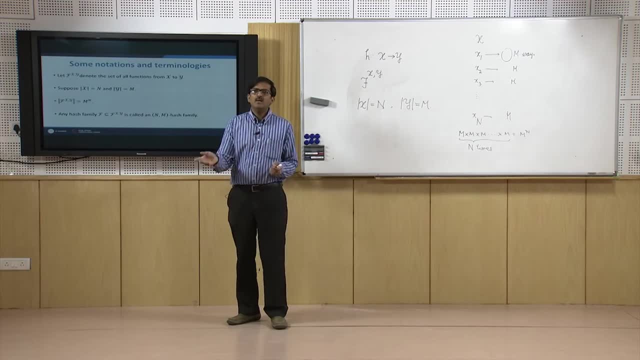 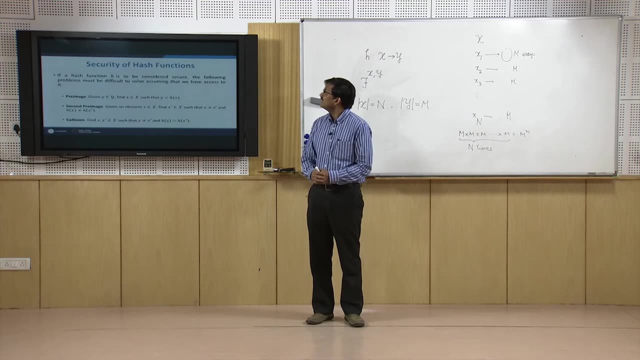 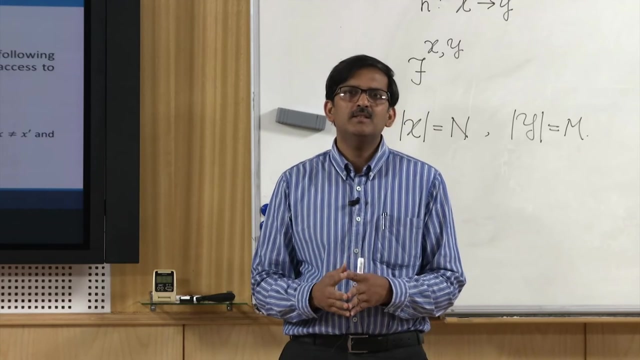 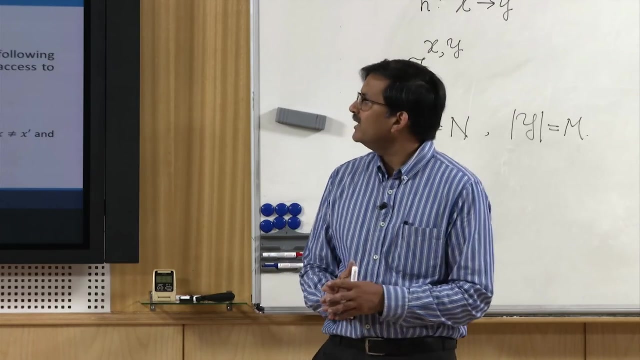 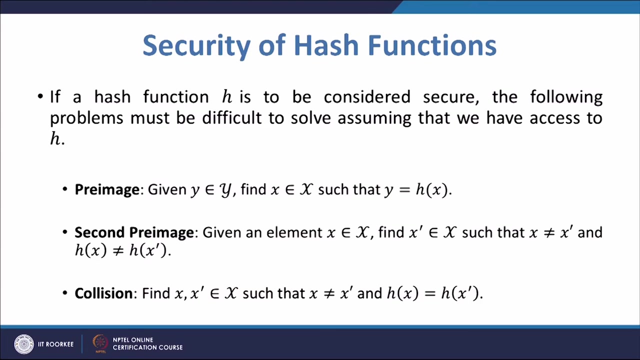 of f, x, y and these are called n, m hash families. So last topic that we discuss in this lecture is security of hash functions. So what has been found is that we have a hash functions must have some properties to be secure and these properties are formulated. 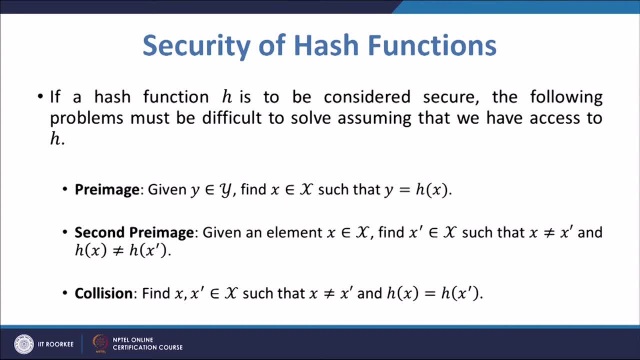 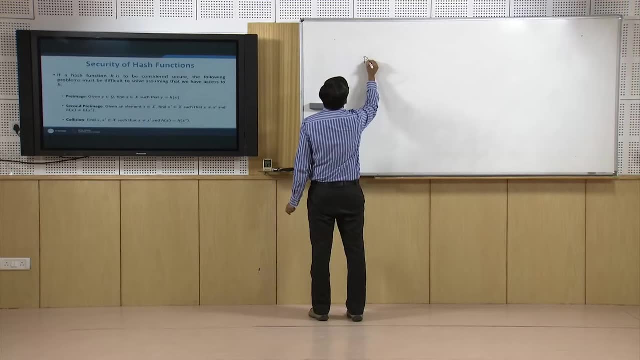 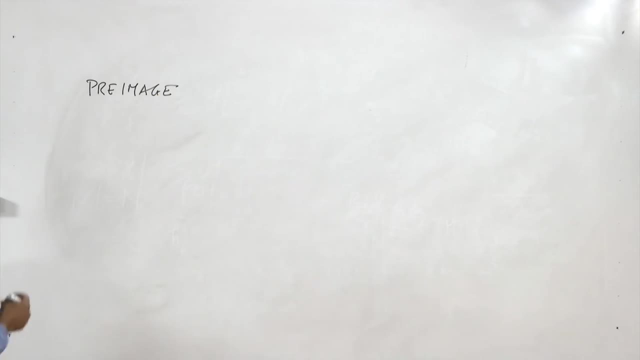 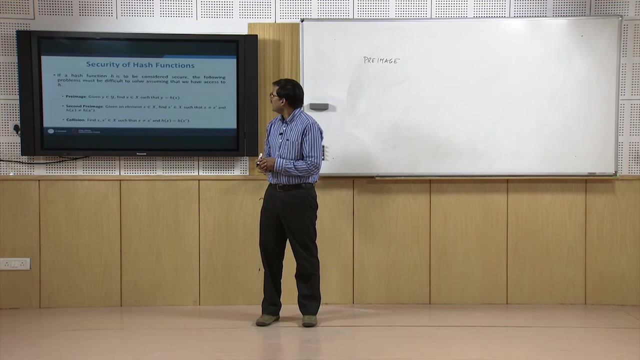 as problems. So these problems are preimage, second preimage and collision. So let us think in this way: we have a problem called preimage. What is that problem? This problem state that I am given something. I am. I have got the access to a hash function. 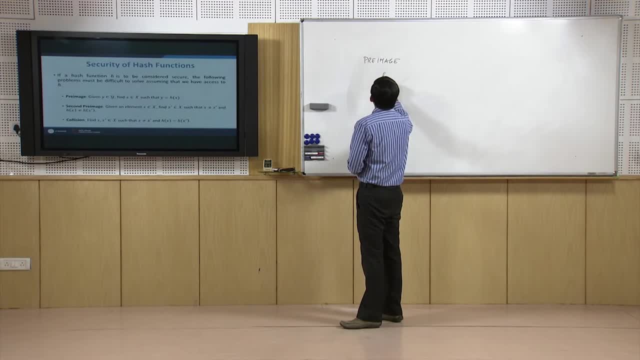 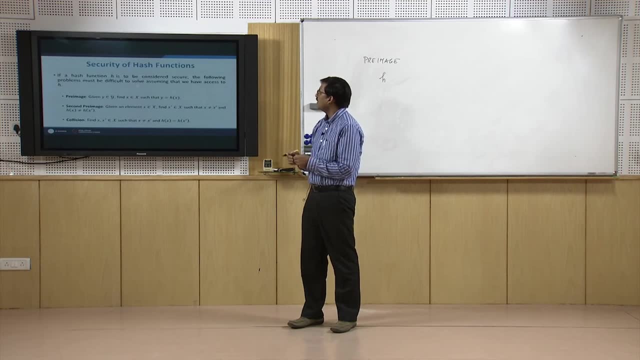 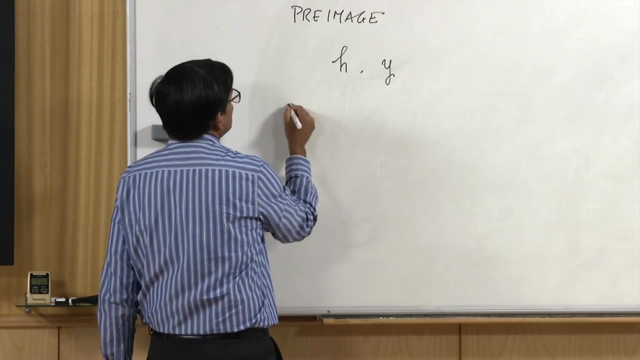 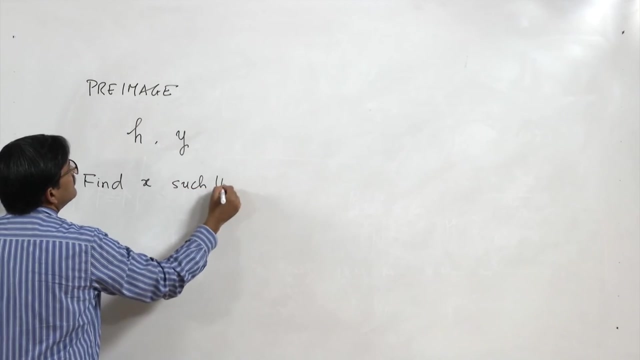 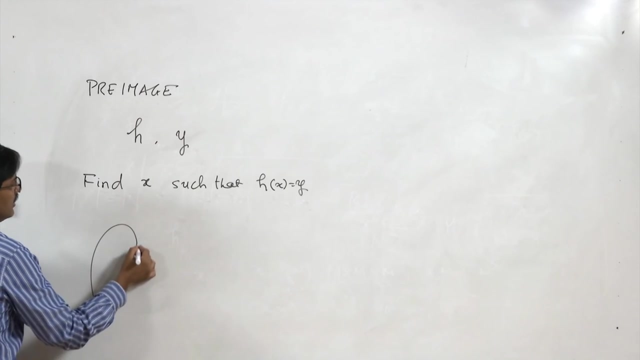 h And I have got. I have been given a, I have been given a y. So these are the things that are given to me and I have been told that find x such that h of x equal to y. So this means that in a way, I got huge space. 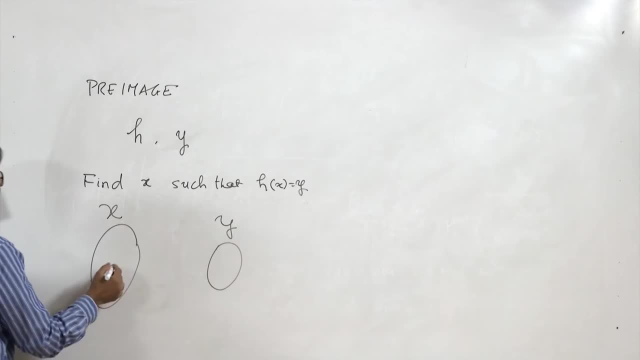 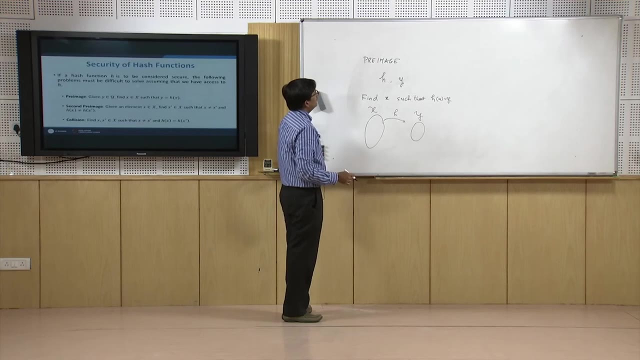 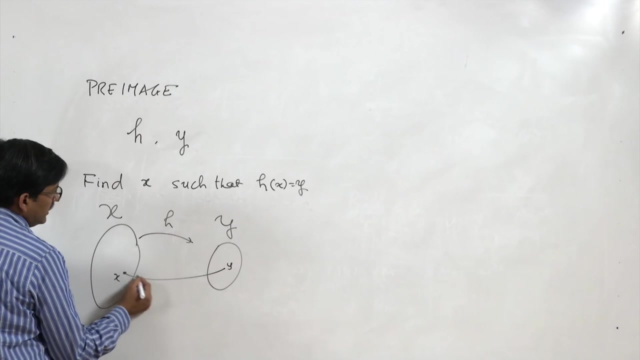 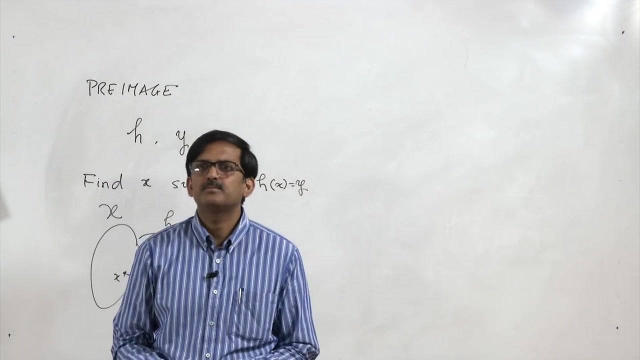 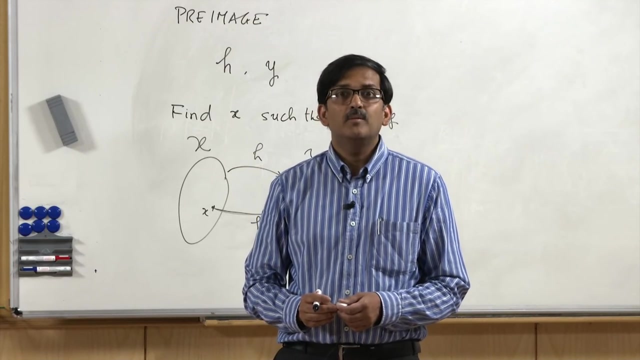 x, smaller set y. and well, I am given the function and I am given a y and I have been asked to find out x, such that x is taken to y. this is preimage. Now, if a hash function has to be secure, then this preimage problem must be very difficult to solve. that is to say, 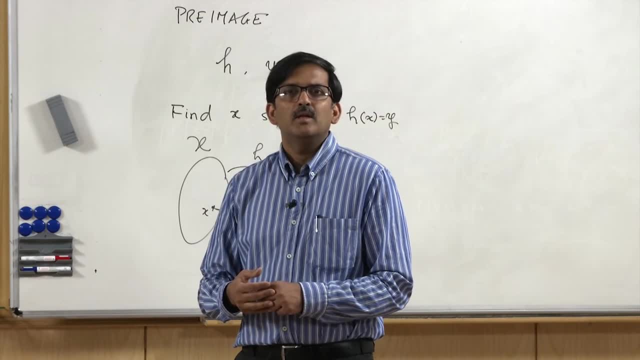 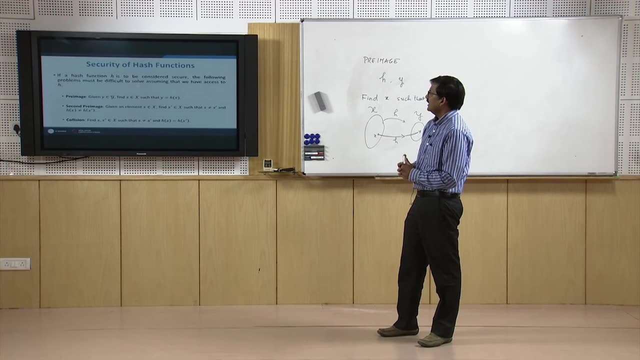 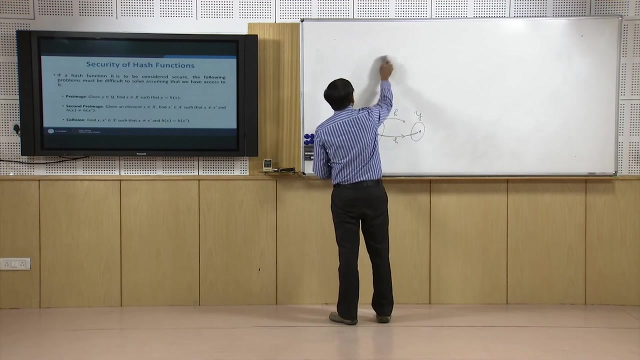 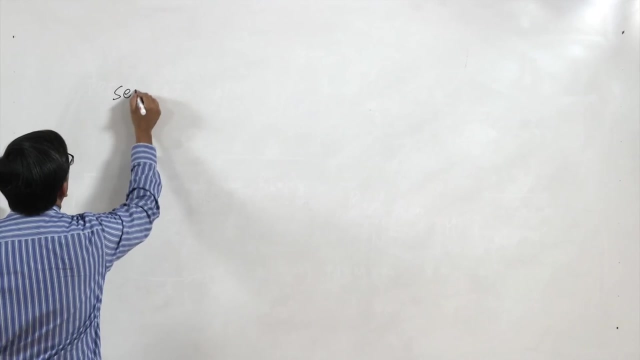 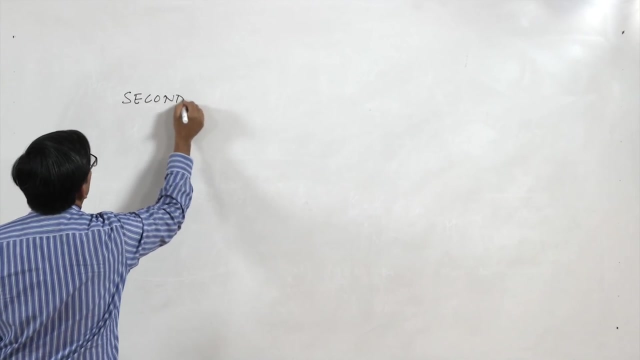 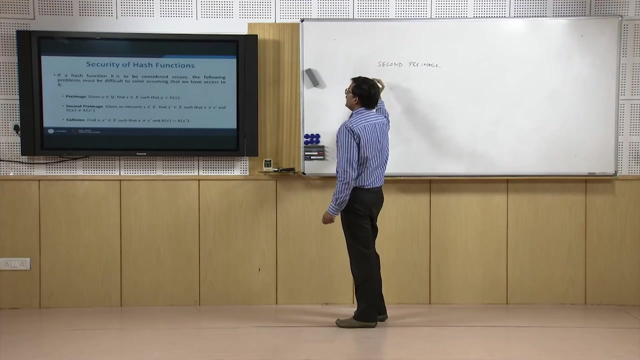 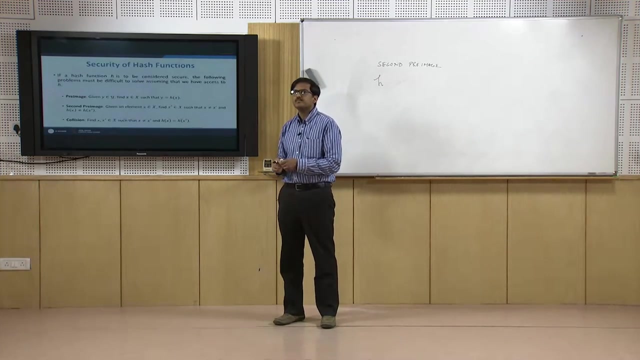 it should not be possible to solve it in feasible time Now. second preimage: second preimage is a problem which looks like preimage but is slightly different from that. here again we have a, we have access to H, the hash function, and here I have been asked to find out y and well, I am given a y and well, I have been asked to find out that this preimage problem must be very difficult to solve. that is to say it should not be possible to solve. that is to say it should not be possible to solve. 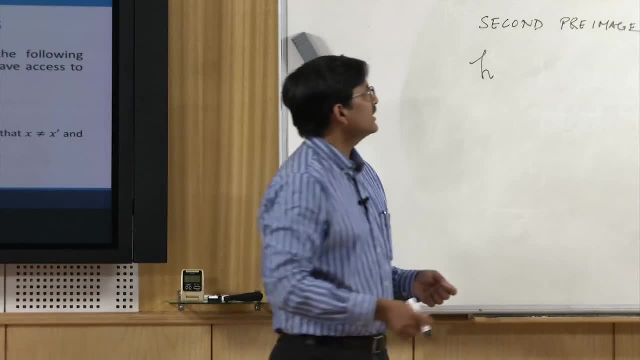 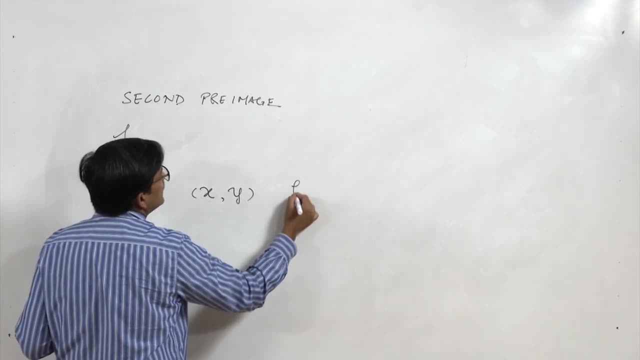 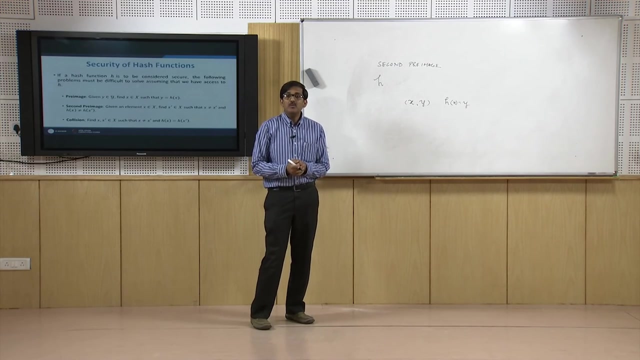 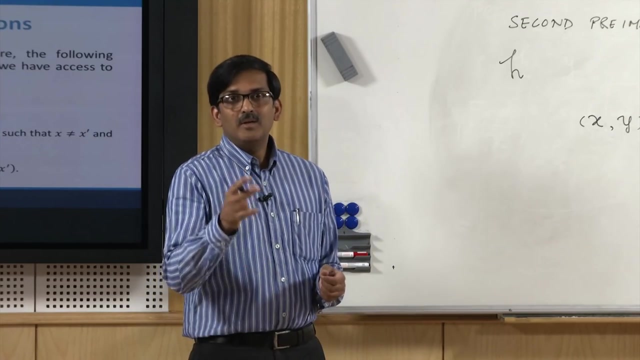 So I have been given a pair, that is, I have been given a pair which is, so to say, valid pair. So I have given a pair such that h x equal to y and I am asked to find out another x. that is a second preimage. we denote it by x prime. 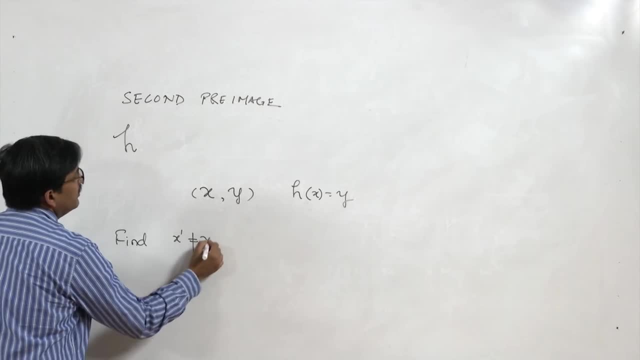 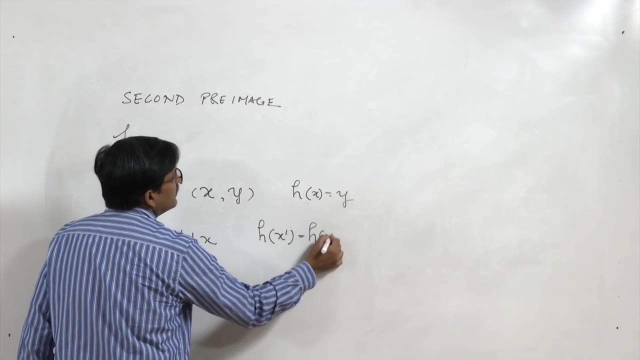 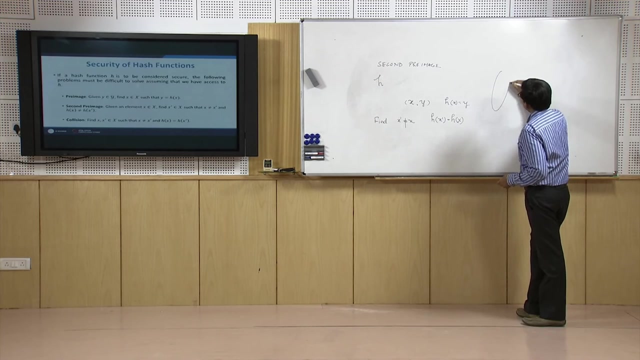 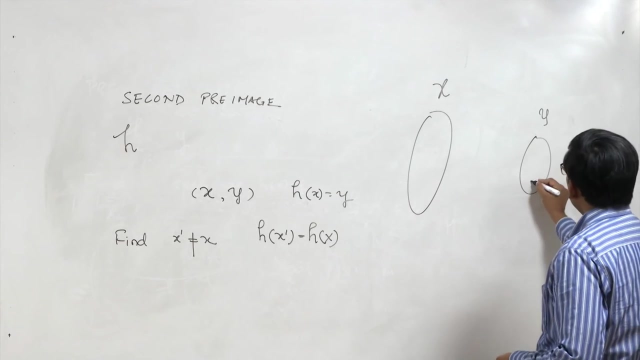 find x prime which is not equal to x, such that h x prime is equal to h x. So if we write a, if we draw a diagram, it will be like this: that again I have this space x and I have this space y. I have been given a y and a pre-image of that, So I know that h x is. 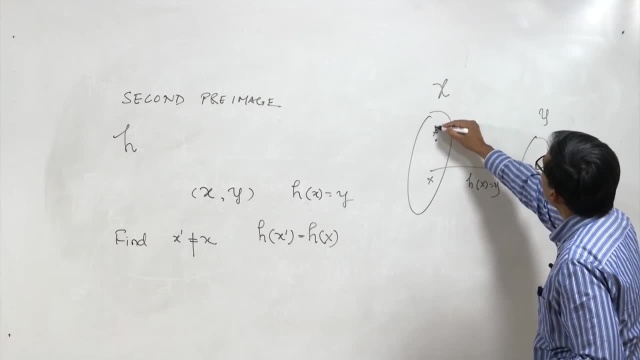 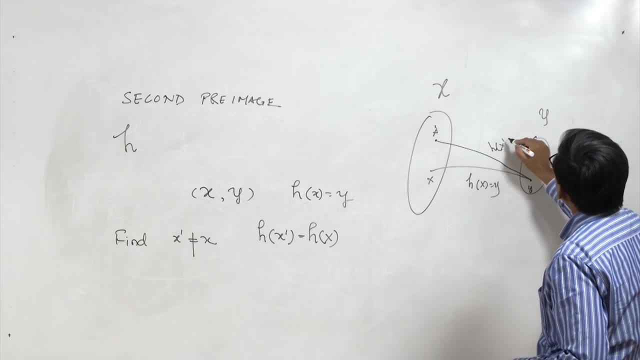 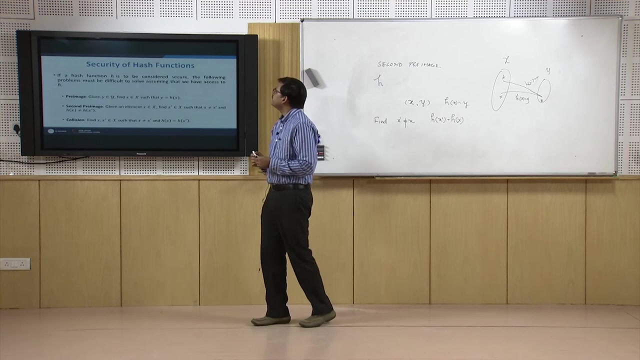 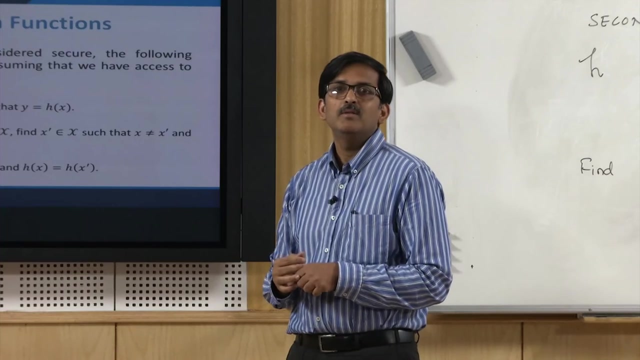 equal to y. I am asked to find something else, some other element in x, such that this also maps to y. h, x dash should be equal to y. So that is the second pre-image. now look at this. lastly, the third problem, which should be difficult to solve or, So to say, practically impossible. 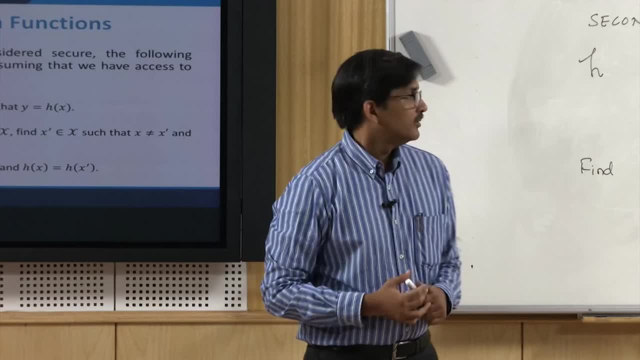 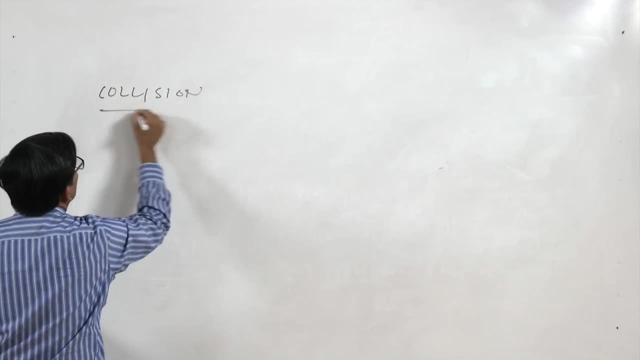 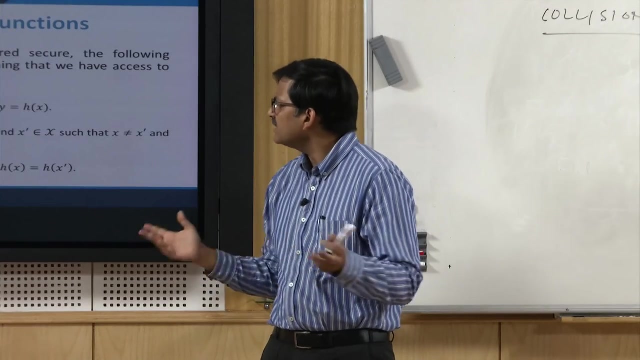 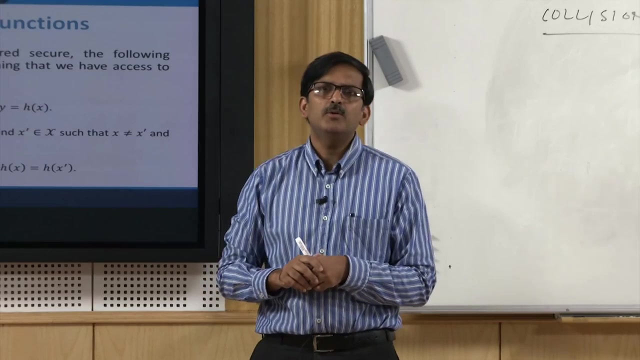 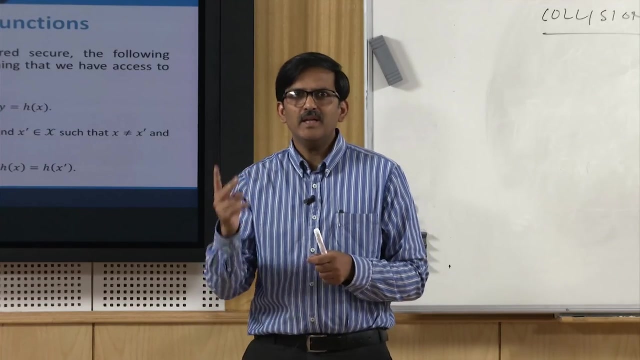 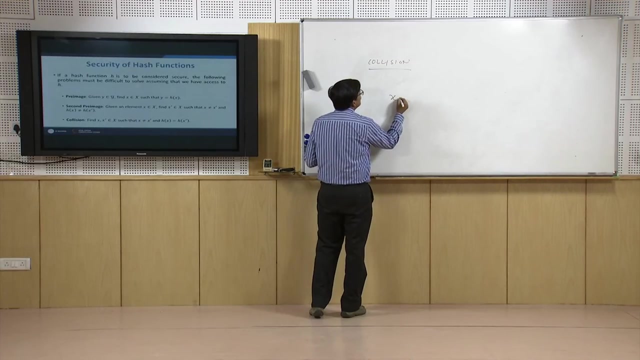 to solve. that is called collision. this says that I have something. I have access to something much less. I have just access to h. I just know the hash function And I should not be able to compute two distinct data sets, x and y. sorry, x and x prime, I should. 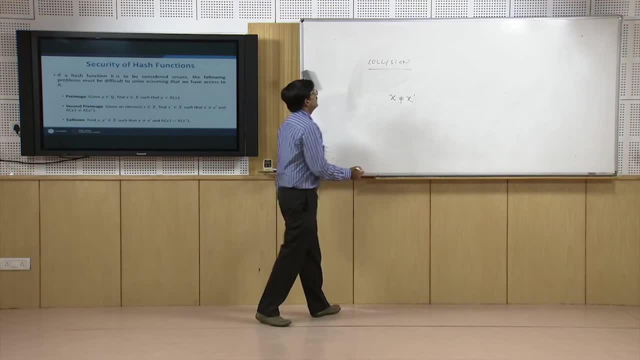 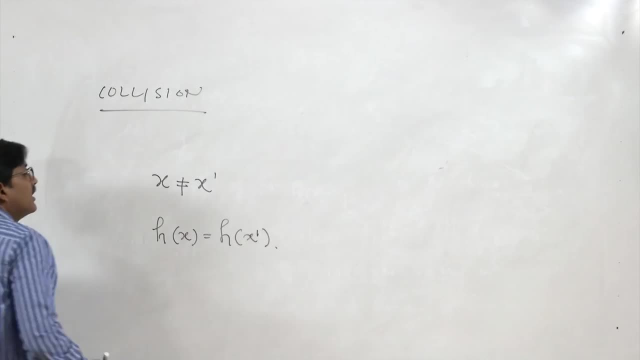 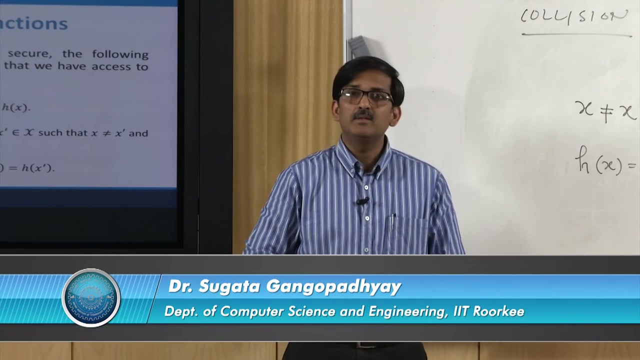 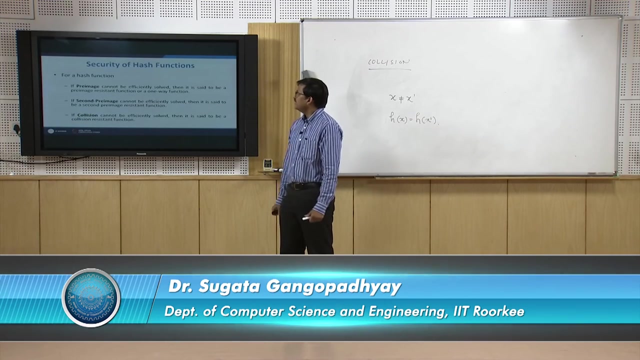 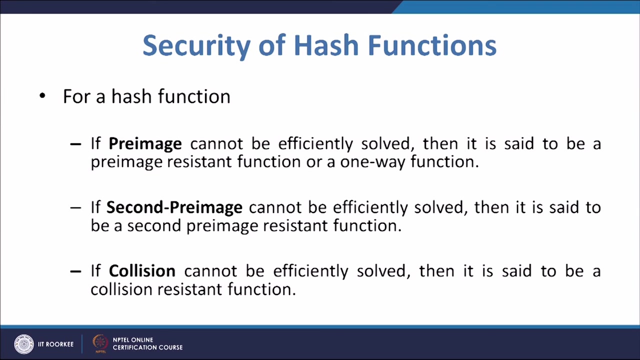 not be able to find x and x prime, which are distinct, whose hash values are same. if I am able to do that, That means that I have got a collision. but I should not be able to do this. so that is collision now at the end, if for a hash function it is not possible to find, or if it is not. 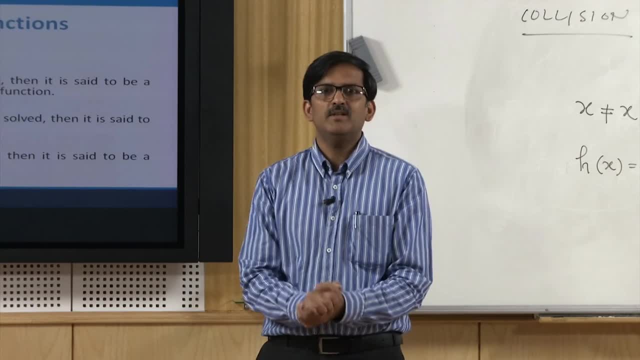 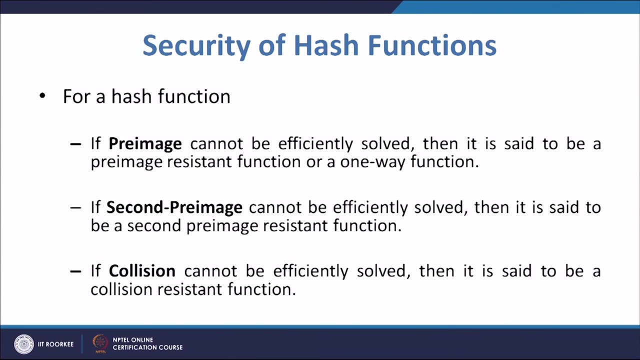 possible to solve pre-image problem, it is called pre-image resistant hash function. If for a hash function it is not possible to solve this pre-image problem, then what we possible to find second preimage, then it is called a second preimage resistant hash function. And lastly, if for a hash function it is not possible to find a collision, it 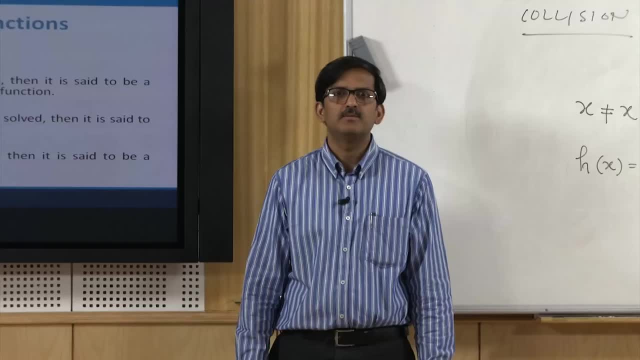 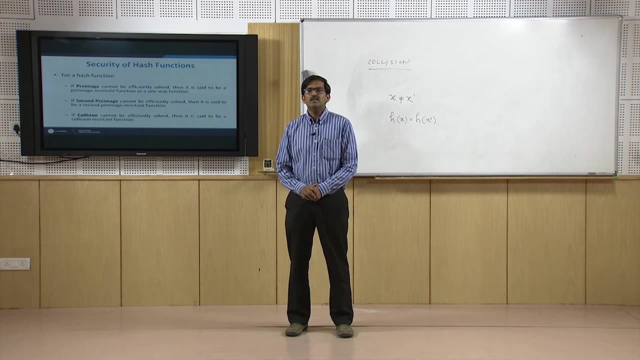 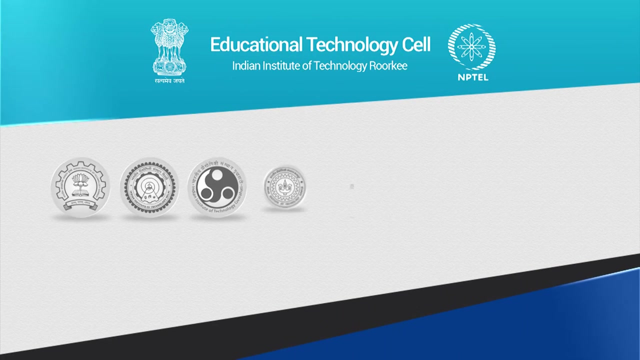 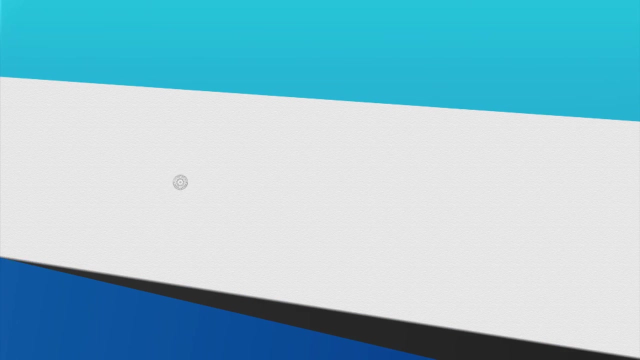 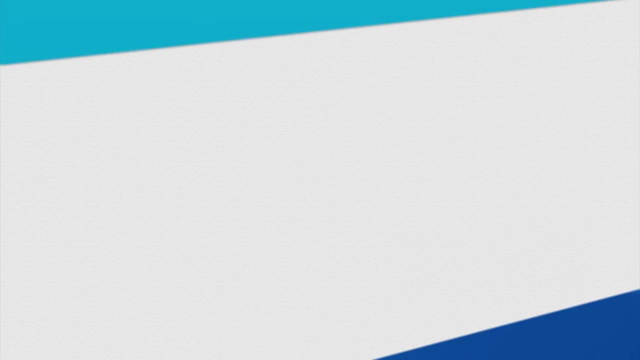 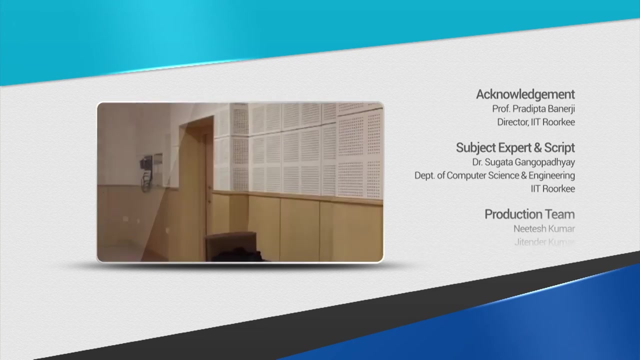 is called a collision resistant hash function. We end today's lecture here. we will consider these properties in details in the forthcoming lectures. Thank you, Thank you.